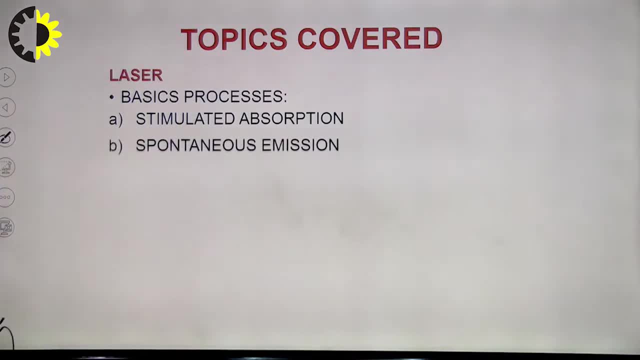 processes involved. The first one is stimulated absorption, then we have spontaneous emission, then stimulated emission. We will discuss all these three processes here. These three processes will be discussed: stimulated absorption, spontaneous emission and stimulated emission. Then I will discuss the principle of laser action, that under the principle under which the light will get amplify. 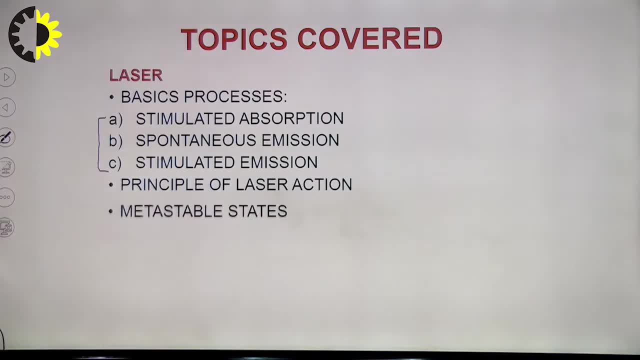 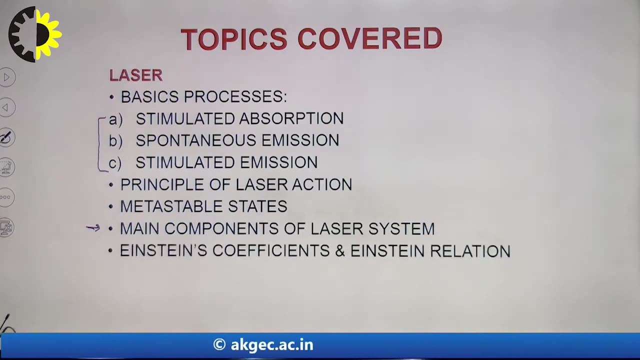 in case of laser. The next topic which I will take, that is, metastable states, and what is the role of those metastable states in case of laser. After that I will discuss the main components of laser, Slide 9.. laser system. Then next one is Einstein: coefficients and the relationship between. 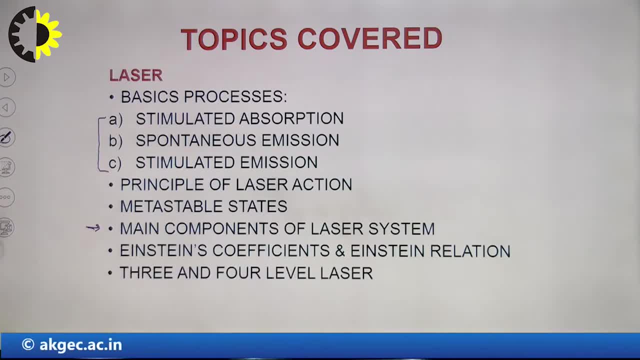 them. After this I will discuss two different type of lasers. First is three-level laser and then we have four-level laser. After that I will discuss two lasers here: Ruby laser, which is a solid-state laser, and then helium neon laser. So all these topics I am going to cover under this heading: laser. 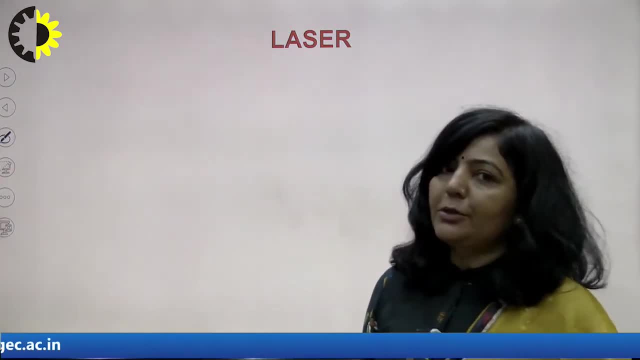 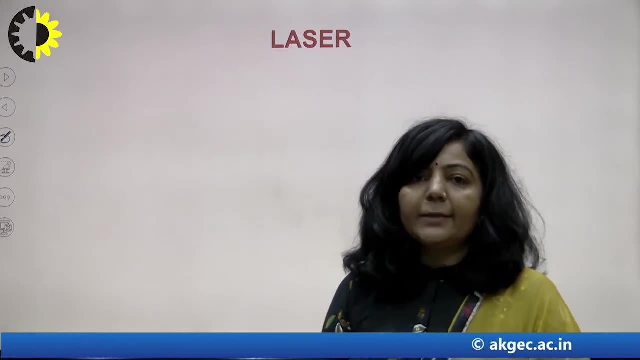 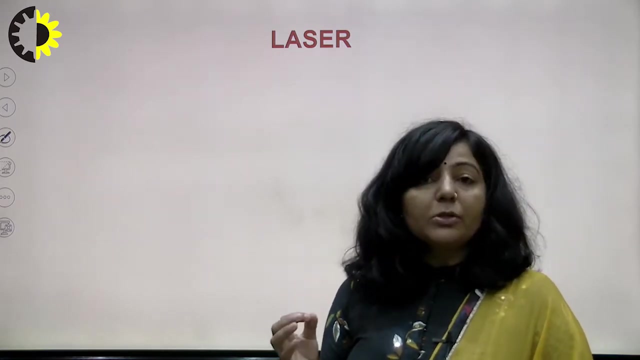 So I am going to start with the basic process or the basic concepts. concept: When I am saying laser, then the first thing which strikes our mind that a highly coherent, highly directional and a very bright light source, And this particular source that is always superior as compared to other light. 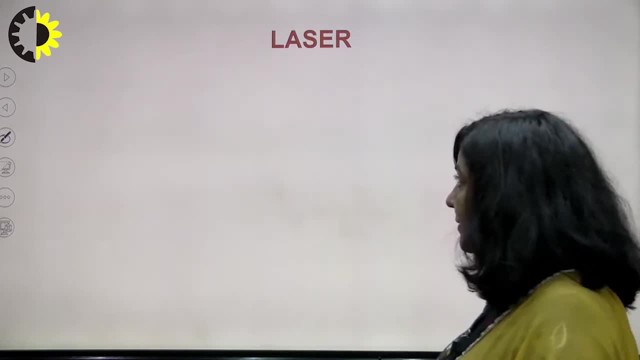 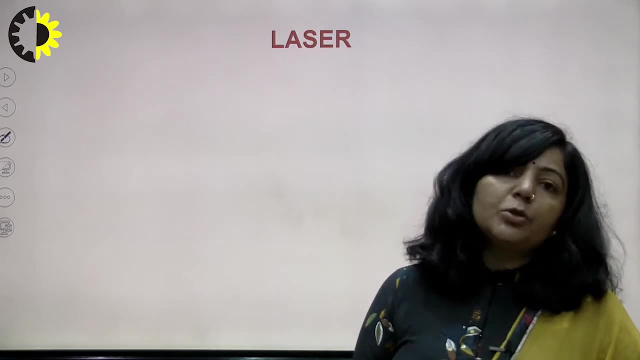 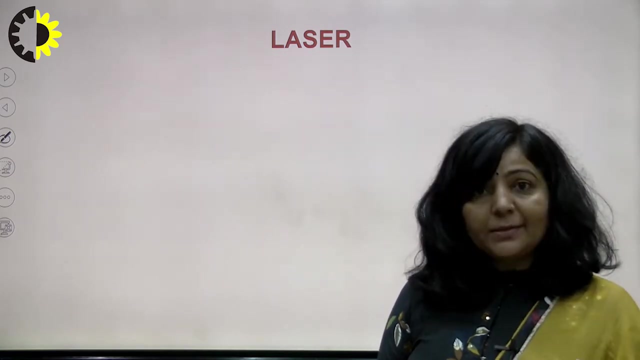 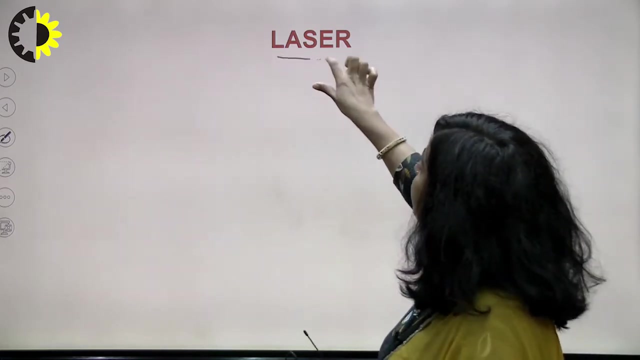 sources or ordinary light sources. Now the question arises that what is the reason or what is that basic process because of which laser is superior as compared to other ordinary light sources? So the reason of that particular reason, of that high intensity, highly coherent nature, highly brightness, low divergence, that lies in this void itself. So this: 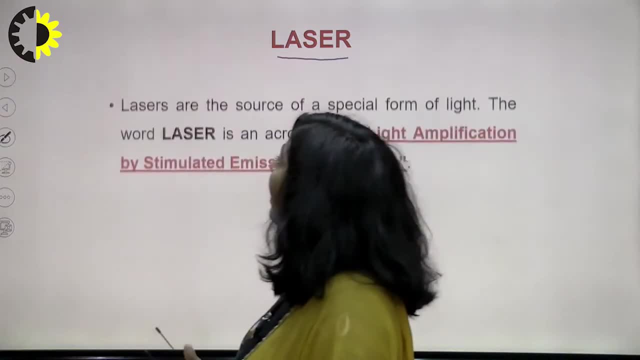 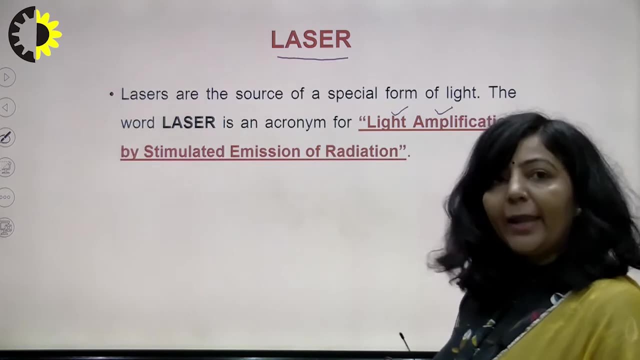 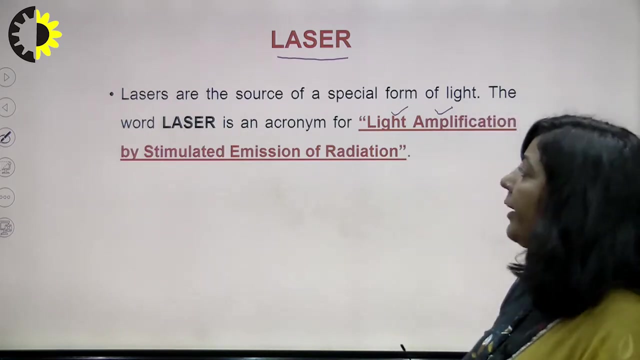 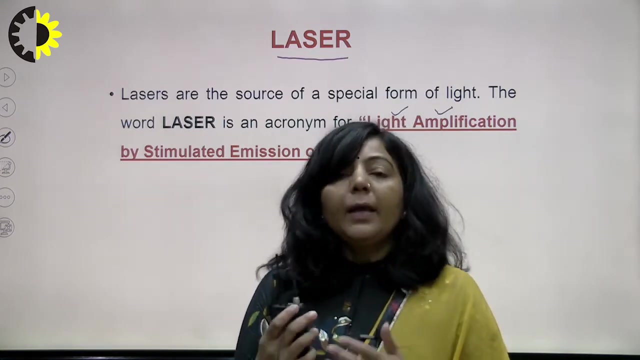 laser. that stands for light amplification by stimulated emission of radiation. this L stands for light, a for amplification and s for stimulator and e for emission. emission of radiation means the entire process that is hidden under this word: laser in case of laser. in case of this. 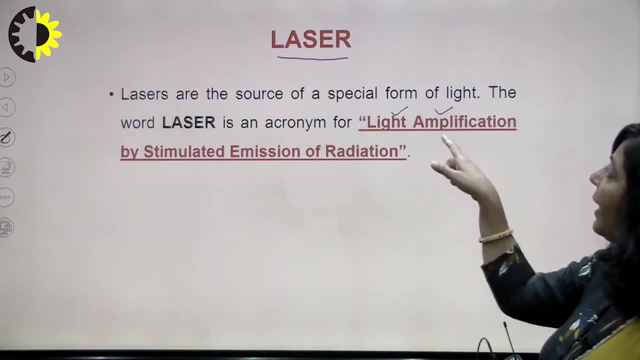 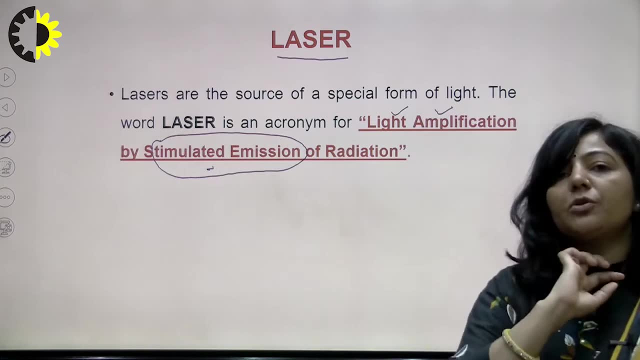 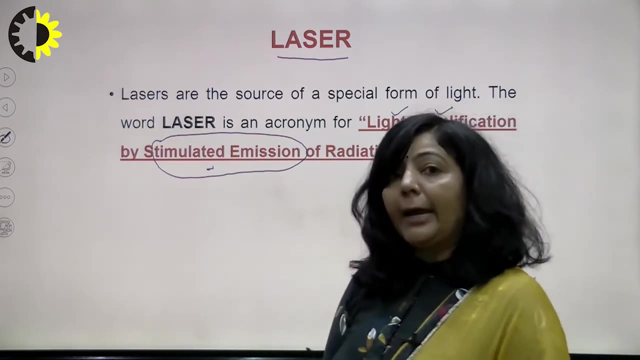 light source. light will get amplified and that will get amplified through this process, stimulator emission. so this process, stimulator emission, is responsible for the amplification of light in a laser source. now we will try to understand that. what is the meaning of this term, stimulated emission? so in 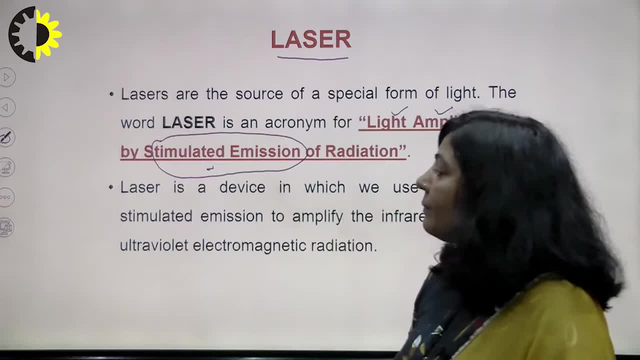 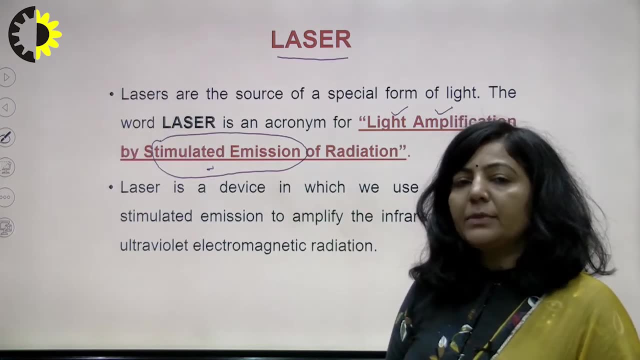 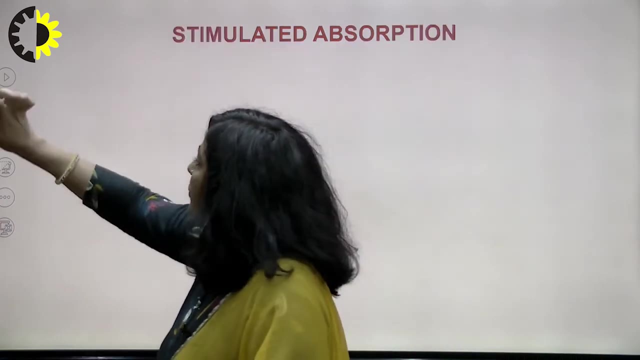 order to understand that stimulated emission, we have to understand that when you are providing energy to an assembly of atoms, and what are the different transitions between these two energy sources and what is the time period in possible in that assembly. So, in order to understand that what I am going to do here, I am going to take an assembly. 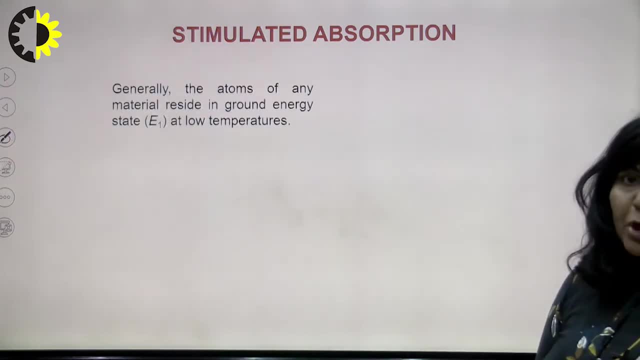 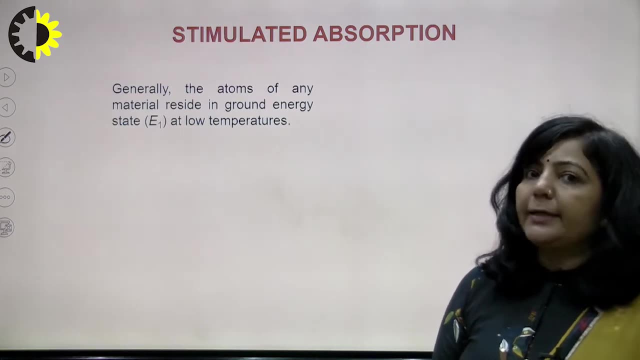 of atom. I am going to start with this process, stimulated absorption. Basically, there are three processes which are equally involved in the amplification of light: in laser: Stimulated absorption, then you have spontaneous emission, then stimulated emission, As I have told you that stimulated emission is responsible for the light amplification. 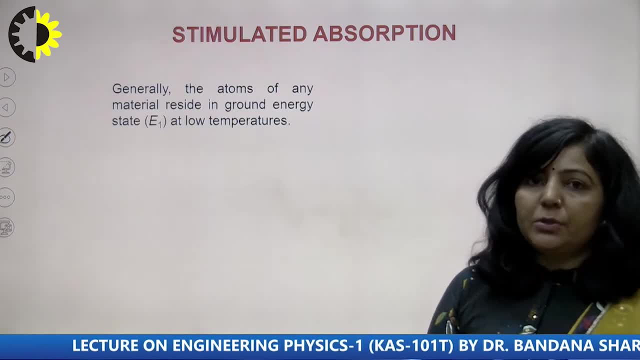 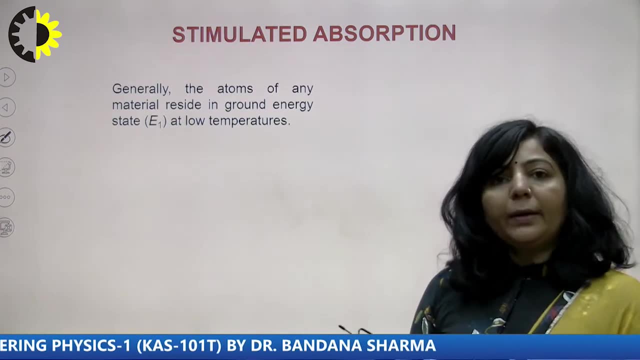 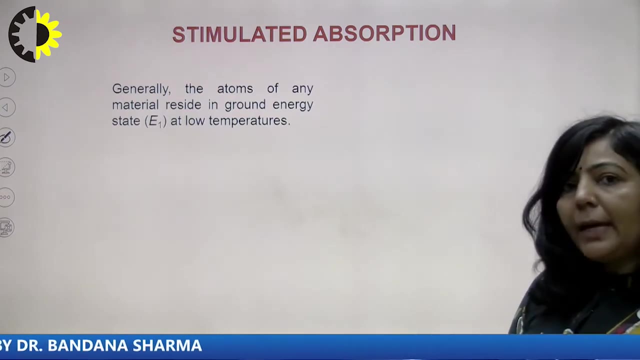 in laser, But without the remaining two processes, we cannot amplify light in case of laser. So it is equally important to understand all the three processes. So I am going to start with this stimulated absorption. So, in order to understand this stimulated absorption, what I am doing, I am taking an 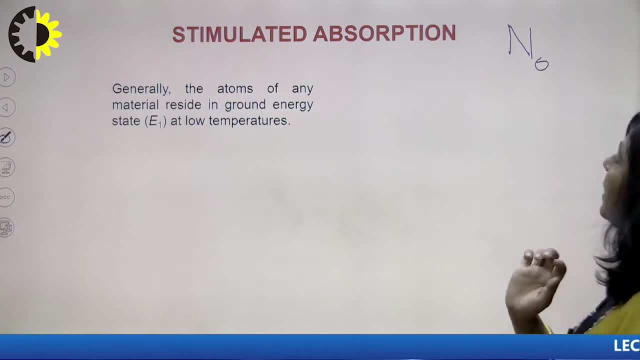 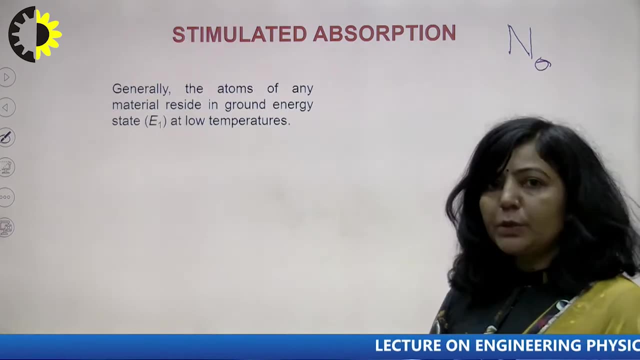 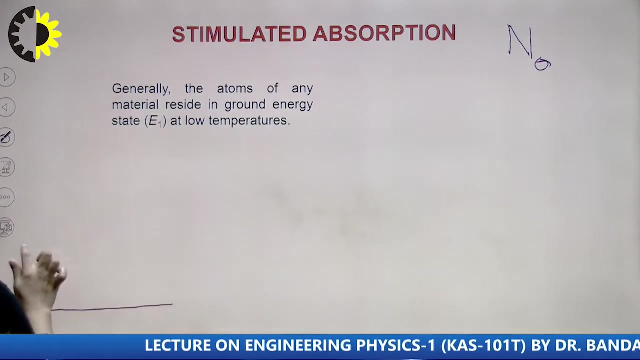 assembly of atoms. So we have an assembly of atoms And in that assembly we have these NO atoms And these atoms, they are distributed in two states. So there are two states in which these atoms can exist, State number 1 and state number 2.. 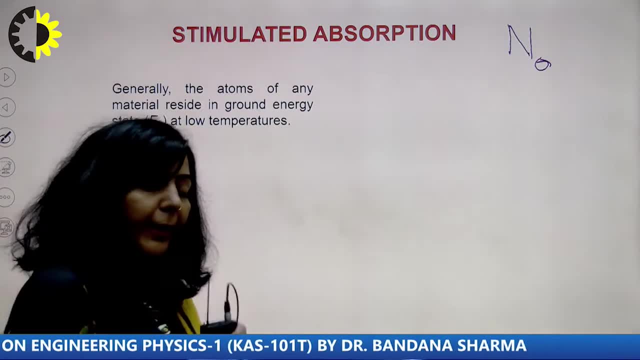 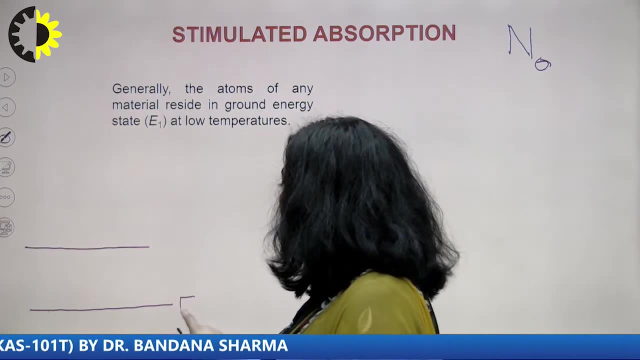 So this state, number 1, that is a ground state, It is having lower energy, least energy in this assembly of atoms, And let the energy of this state is E1. And this is the high energy state in which atoms can exist. 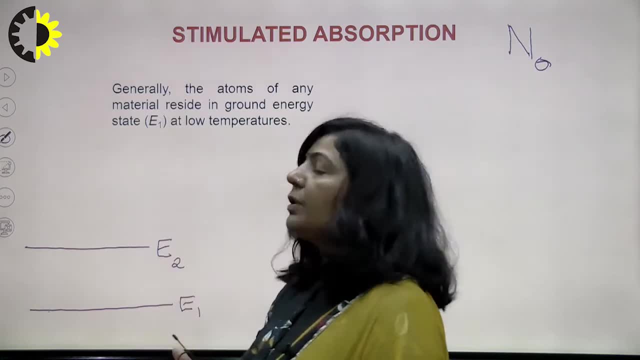 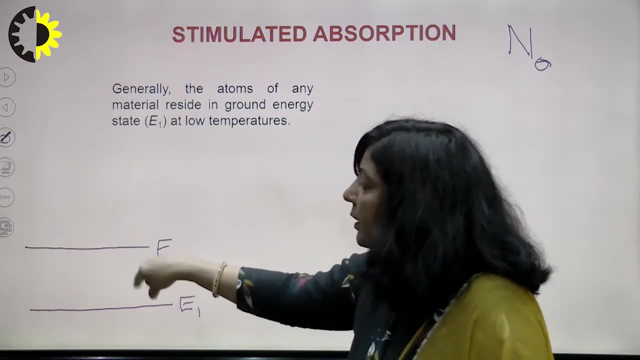 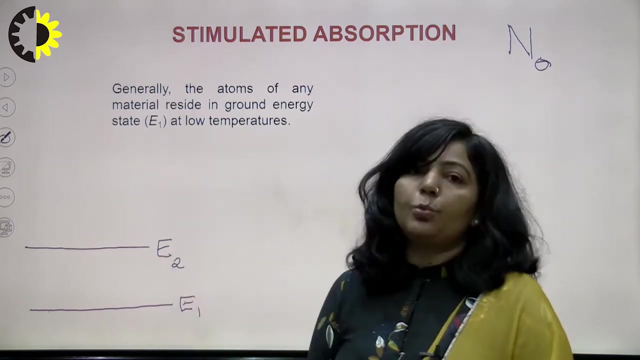 Let. E2 is the energy of this particular state. So these are the two possibilities. You have two states And total NO atoms. they are distributed in these two states. Either they are present in state 1, with energy E1, or they are present in state 2.. 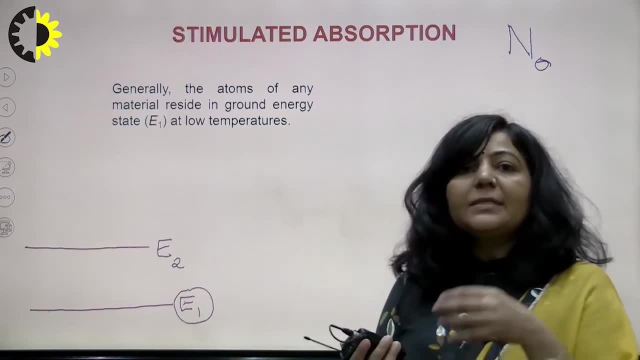 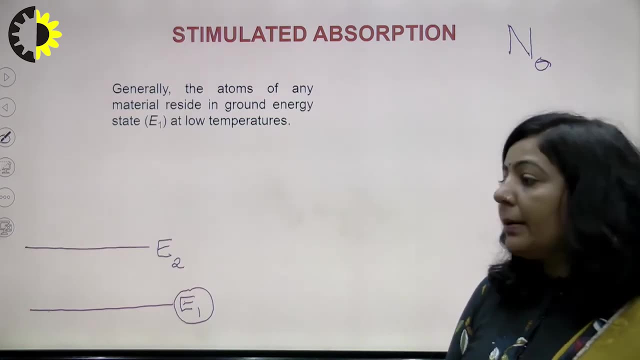 Now this state, number 1, which is having energy E1, this is the lower energy state, This is the ground energy state, That is the energy state And in this state they exists more state and it is the more stable state. 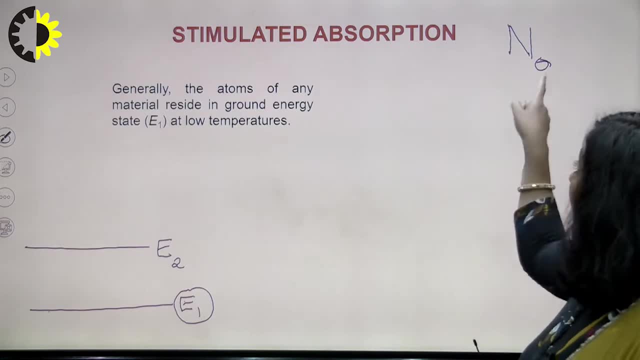 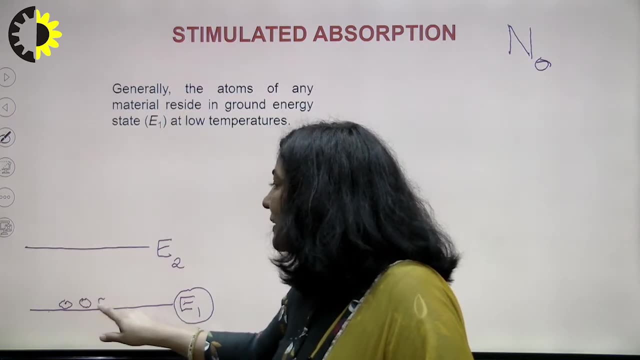 And everything in this universe that tries to remain in a stable ground state. So you can say how, out of these NO atoms, most of the atoms, they are present in this ground state. So these circles, they are representing the atoms of this ground state. 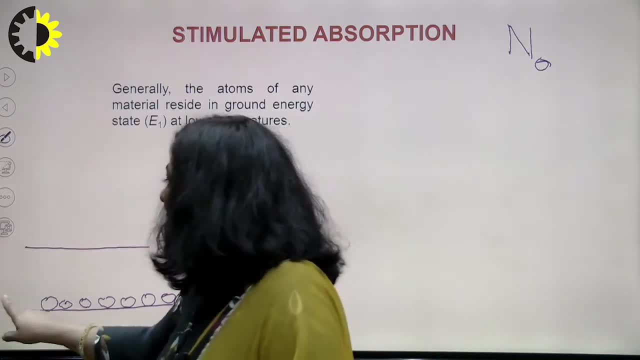 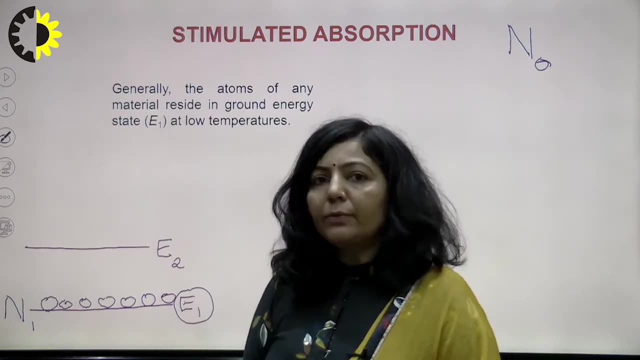 So you can say that, out of NO, most of the atoms are present in ground state, And let the population of these atoms is represented in no state, o represented by n1. so n1 these are the atoms of ground state, and only few atoms. 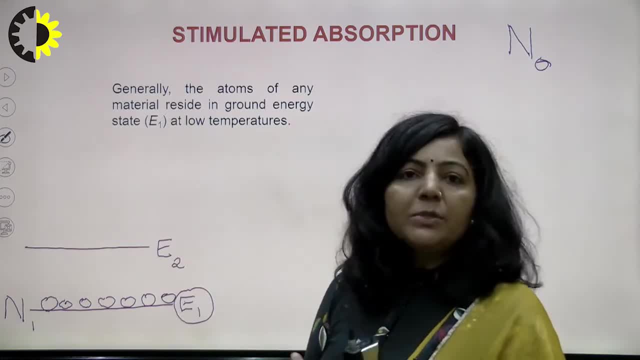 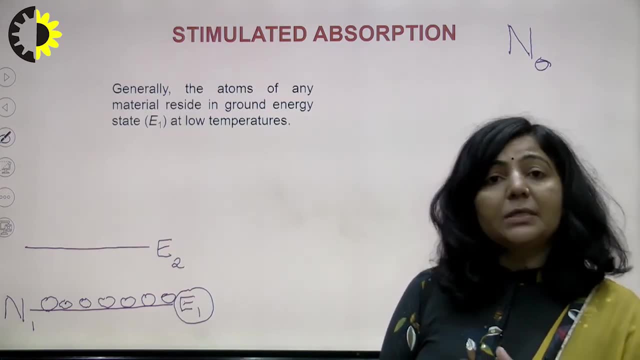 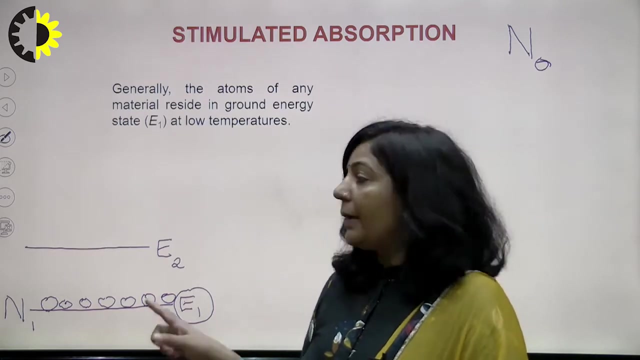 they are present in this excited state. why I am saying few atoms? because this state number two, that is an excited state and it, this particular state, is highly unstable means unstable means the lifetime of this state is not very long. atoms can stay here only for a short duration and that duration is 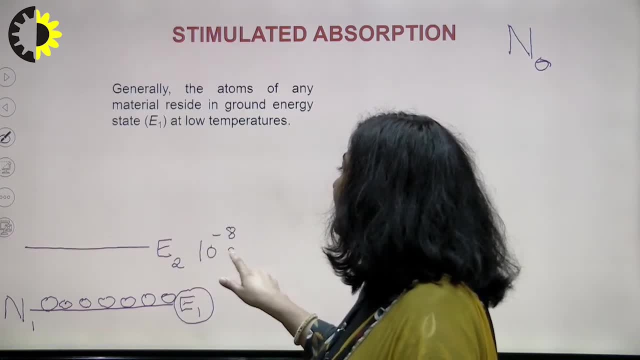 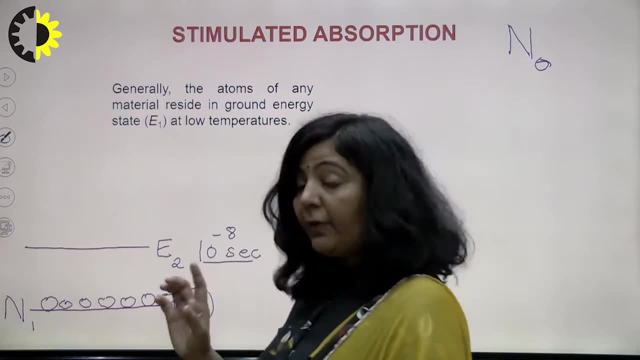 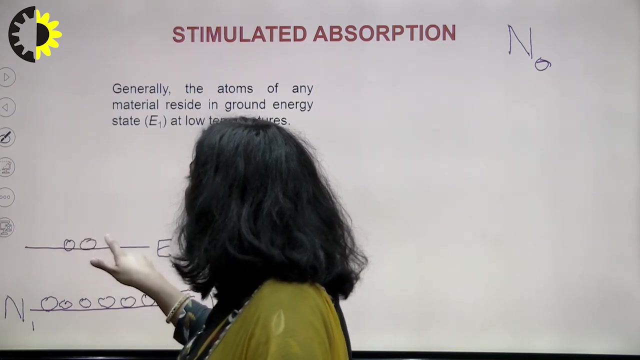 approximately 10 raised to power minus 8 seconds means atoms can stay here only for this short duration. so what will? so what we have now here? we have only few atoms. we have only few atoms here. only n2 atoms are there. so this n2, this 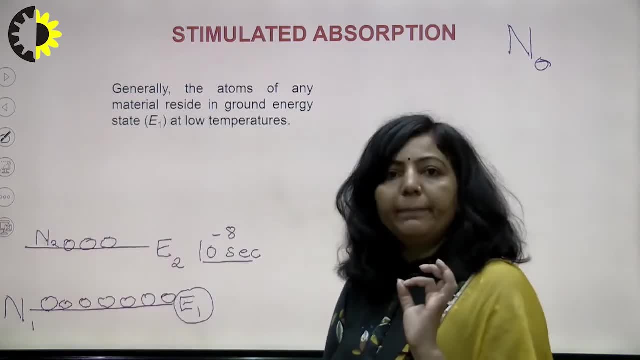 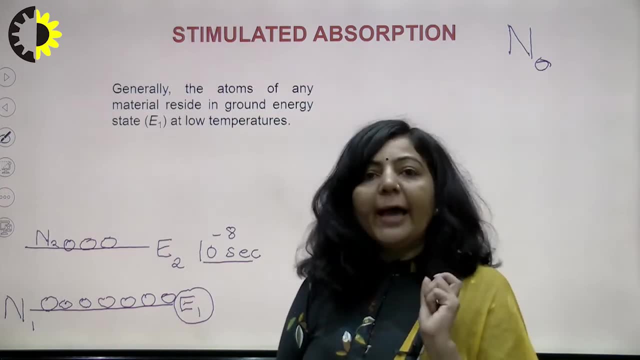 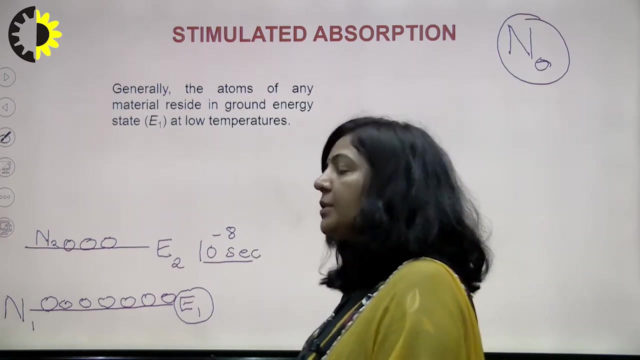 particular population, n2 is very, very small with respect to n1. this is the normal condition. now I am beating this normal condition again. we have an assembly of atoms- you have total and not atoms, right, and these atoms, they are present in two states. we have only. 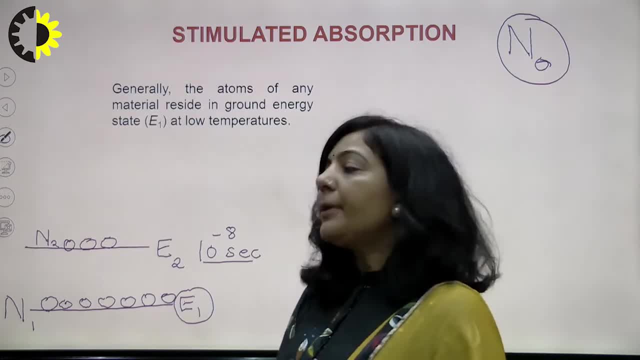 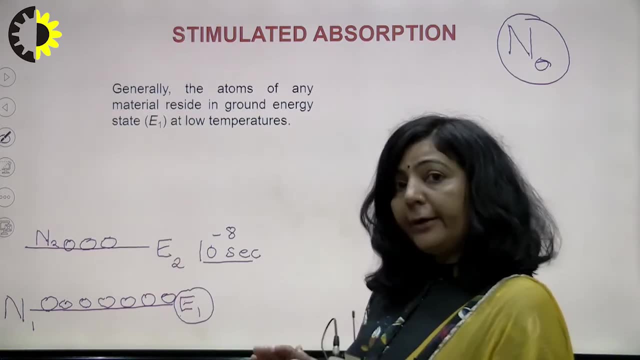 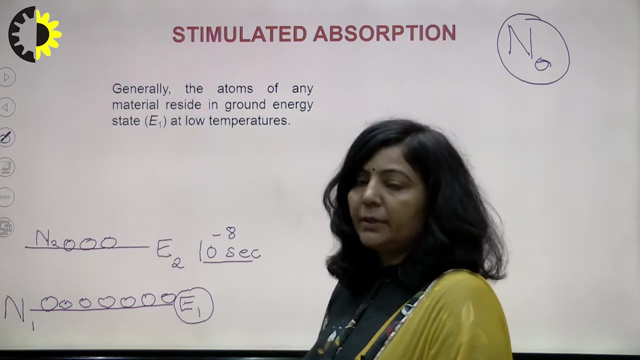 two possibilities for these atoms. either they are present in state one, with energy even, or they are present in state two with energy e2, one. that is a ground state, that is a very stable state. so most of the atoms, they will try to remain in that stable state. so I am. 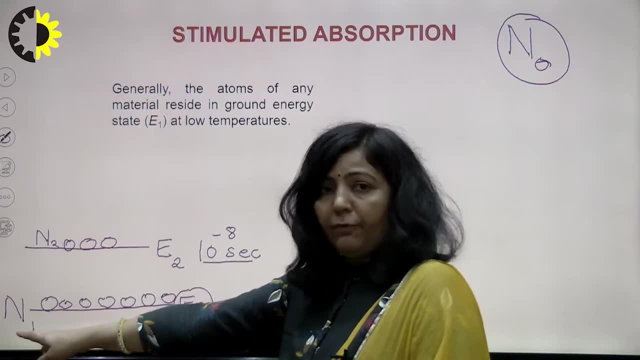 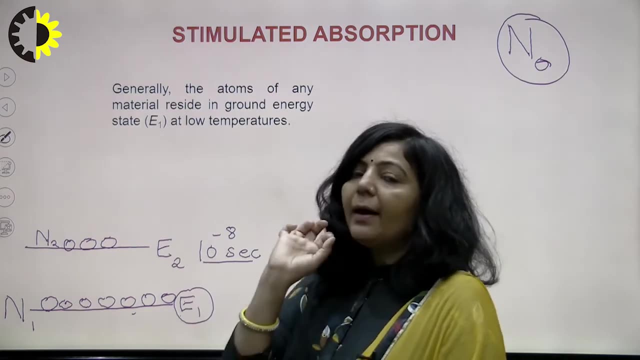 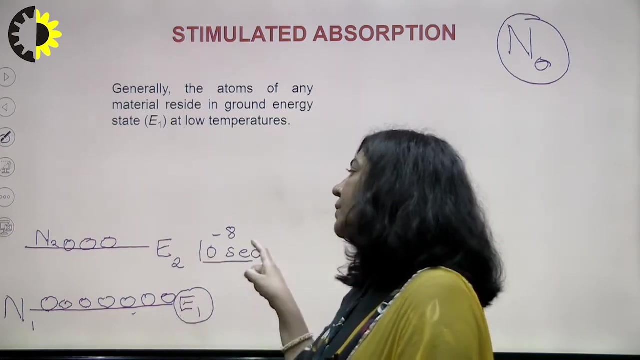 representing the population of ground state with n1 and you have a large numbers of atoms in this particular state state too, that is higher or excited state, and this particular state is highly unstable. why I'm saying unstable? because this state is having a very small lifetime atoms against a. 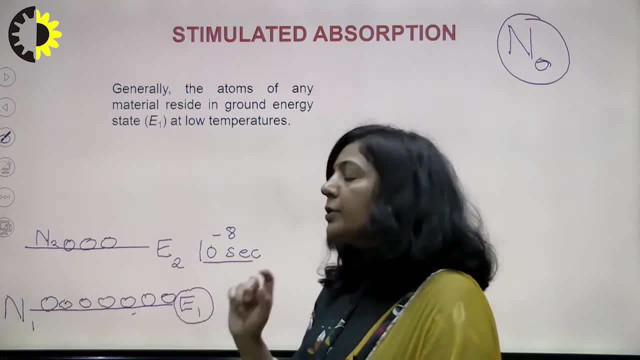 dear atoms can exist in that state only for 10, raised to power minus 8 seconds, and after that automatically novamente тот moments umлен condition'm titan. wird теперь편의 state alive do arsenal will�たppe. They will try to come down to a more stable state. 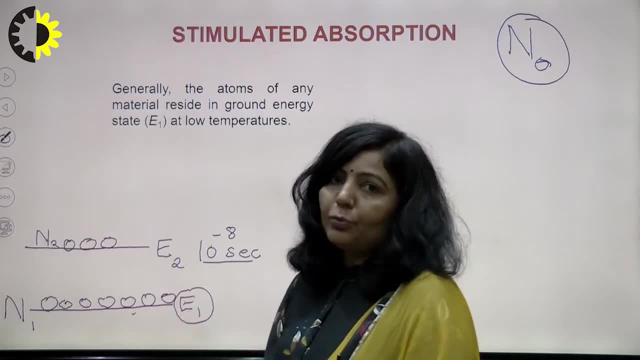 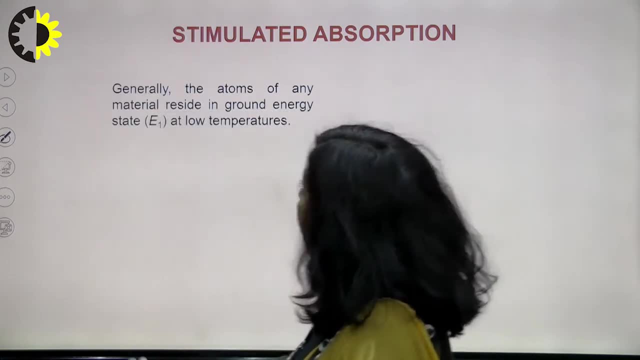 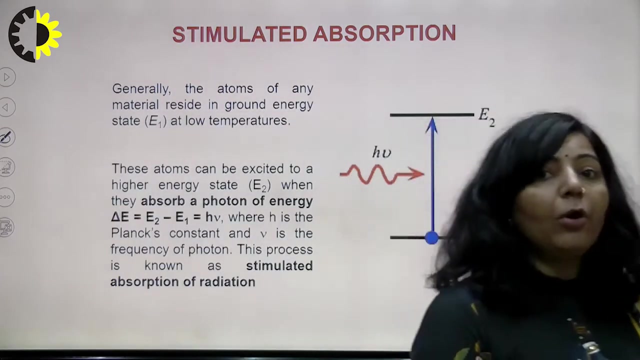 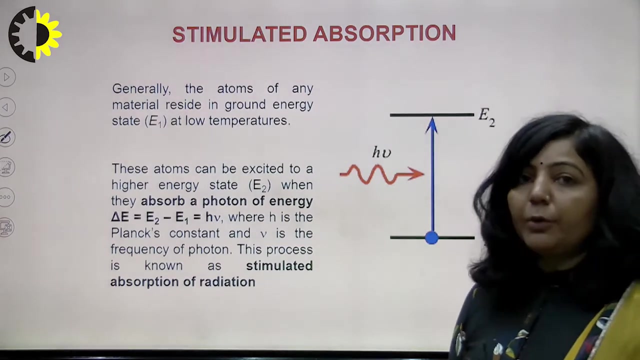 I am representing the population of this state with N2.. So you have this particular case here Now, in this assembly of atoms, where you have NO atoms distributed in 2 states. Now we are providing energy to this assembly of atoms, What you are doing now. 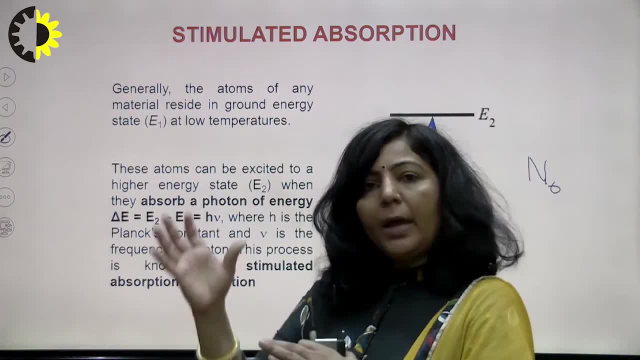 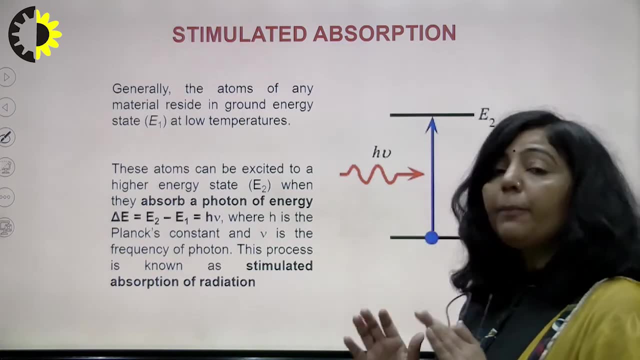 You have total NO atoms there: N1 in ground state and N2 in an excited state. Now we are giving energy to this assembly of atoms from an external source. So when you are providing energy to that assembly of atoms from an external source, 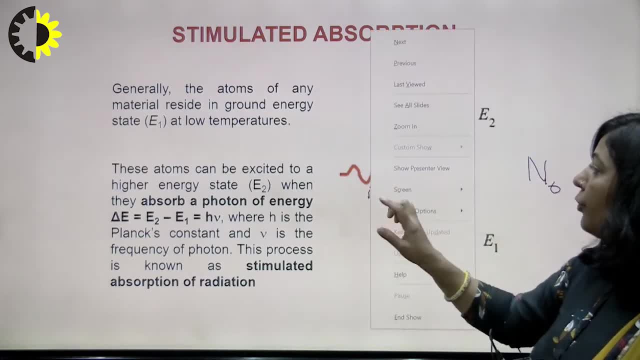 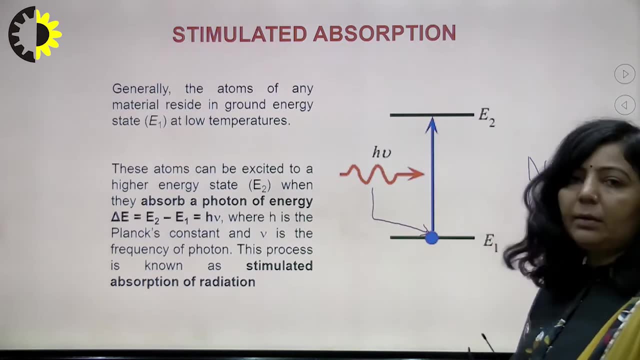 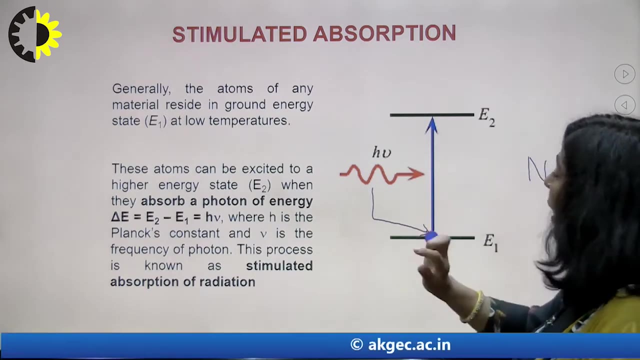 Then that energy which is provided in the form of photons- Sorry, This energy is provided in the form of photons. Now, the atoms which are there in ground state, They can absorb these photons After absorbing this photon, And you have to take this point into consideration here. 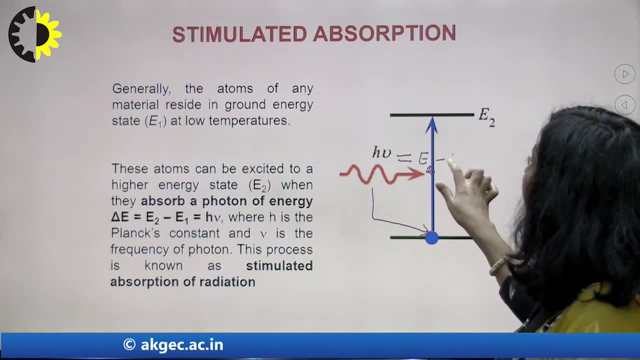 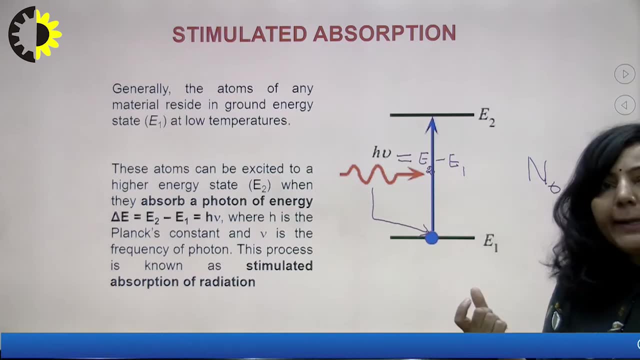 That the energy of this photon That is equal to E2 minus E1. Energy difference between these two. If we are providing photons, If we are providing energy Equal to energy difference between these two, Then that photon will be absorbed by the atoms present in ground state. 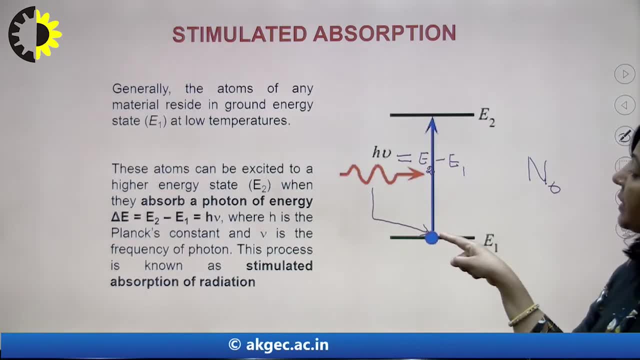 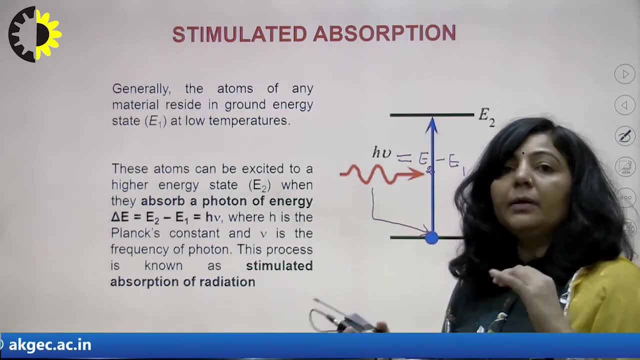 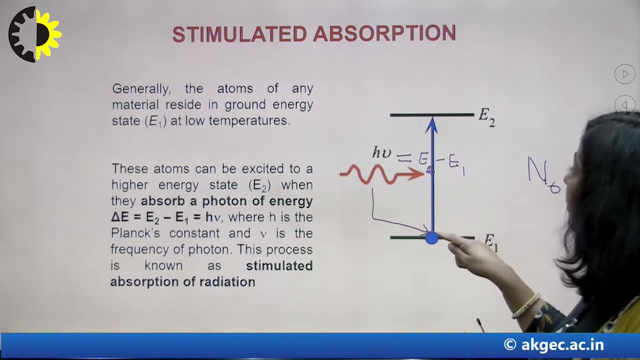 And after absorbing that, photon Atoms can move From state number 1 to 2.. So exactly what has happened here? Atoms of ground state. They have absorbed the energy. So after absorbing, There is a transition from state number 1 to 2.. 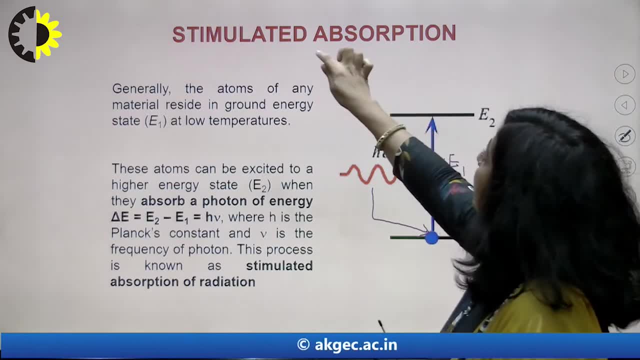 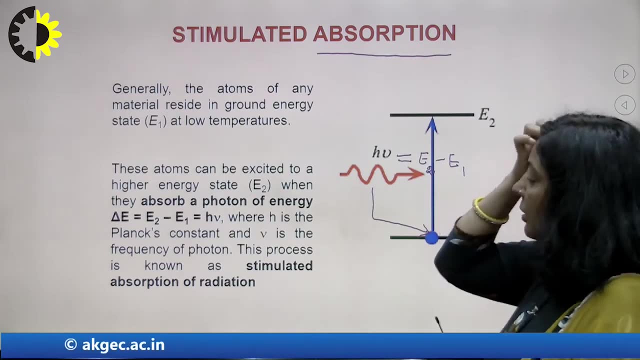 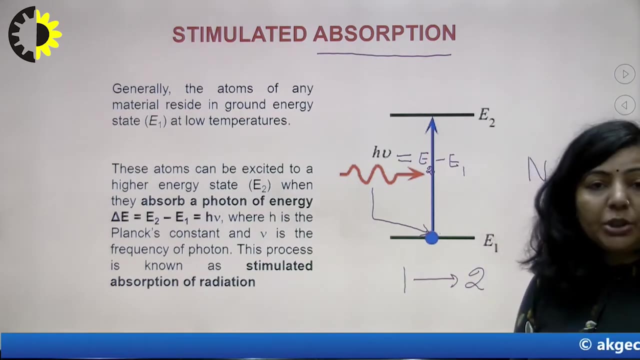 So, since energy is absorbed. So that is the reason This transition, This process is known as absorption process- And since this transition from 1 to 2.. You have a transition From state number 1 to 2.. Since this transition, 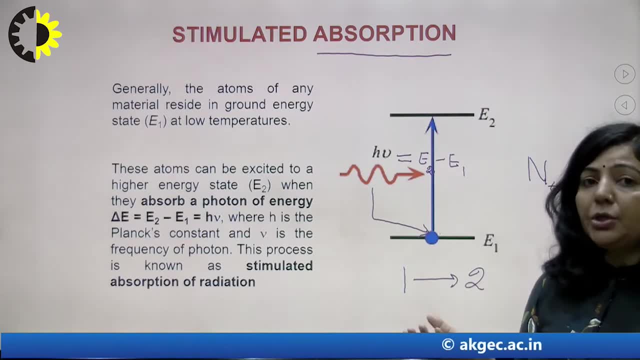 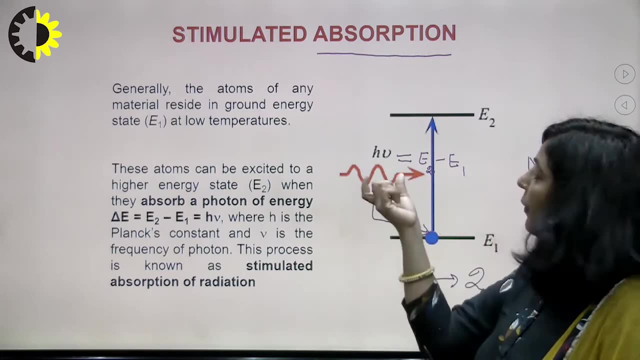 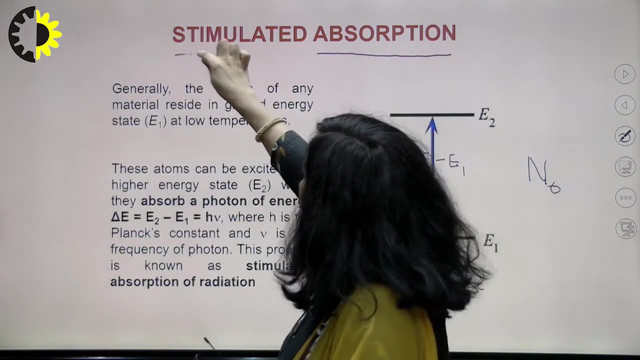 Cannot take place automatically. For this transition, You always require a stimulation, You always require a trigger, You always require a photon Of energy equal to the difference of energy between the two states. So that is the reason This process is known as stimulated process. 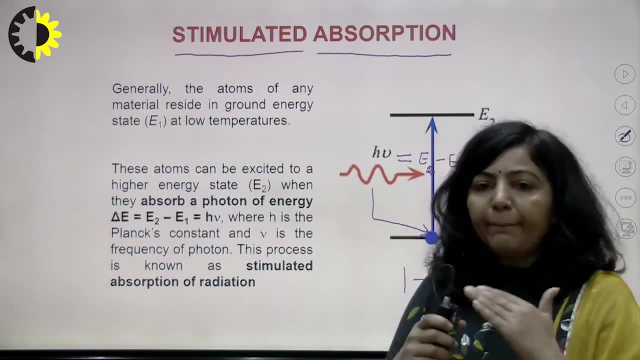 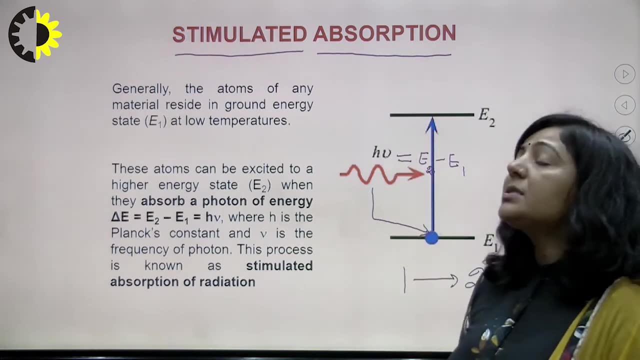 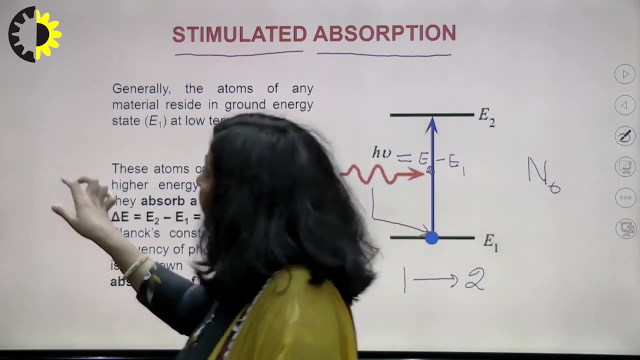 So you have to remember here That absorption is not a complete word, Complete process. Absorption is always a stimulated process, So this process is known as stimulated absorption process. I hope this is clear now. Now, after stimulated absorption, The next process which is involved here: 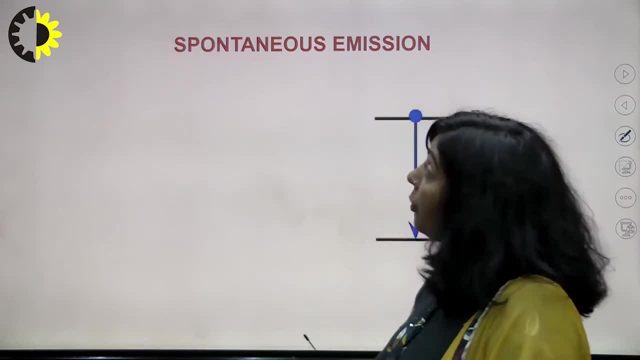 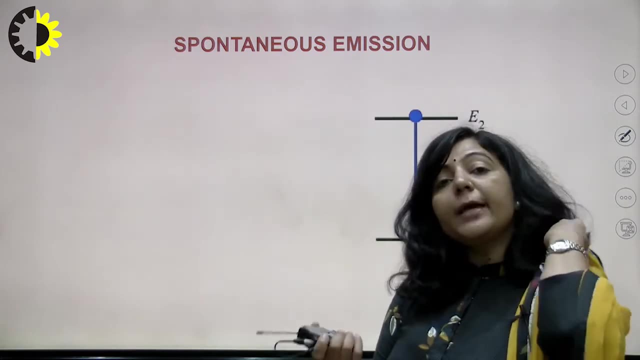 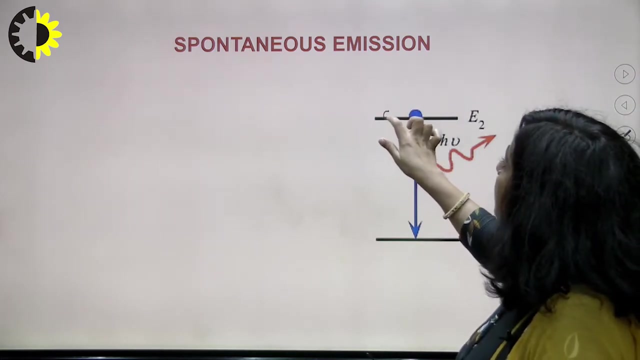 That is, after this, The next process which I am going to discuss here, That is spontaneous emission. So first we will try to understand The meaning of this emission word or emission process. So what we have here? We have N2 atoms in this excited state. 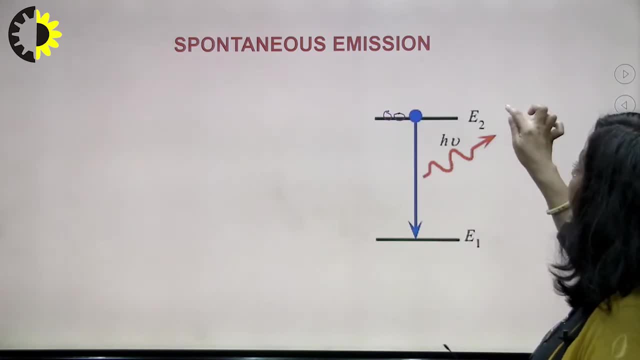 So you have N2 atoms here And you also know That the lifetime of this state- That is also very small, The lifetime is 10, raised to power minus 8 seconds, Means these atoms- Sorry, These atoms- They can stay in this particular state. 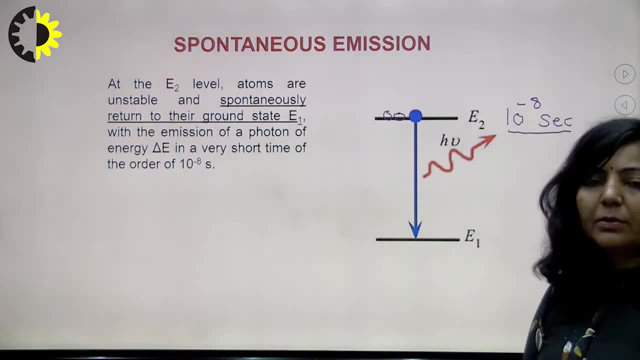 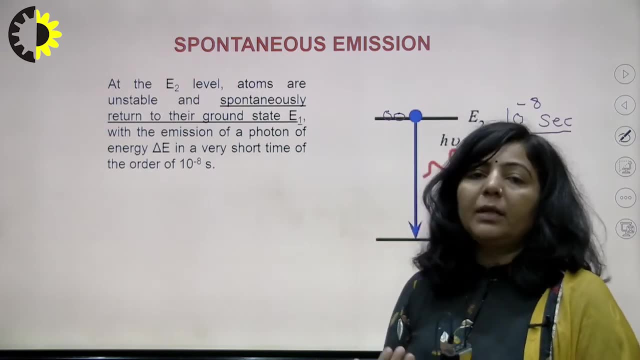 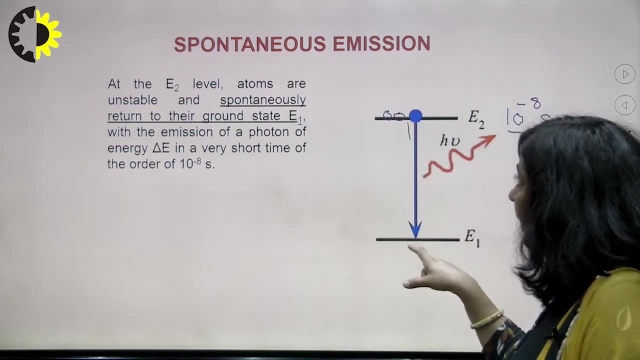 Only for 10 raised to power minus 8 seconds. After 10 raised to power minus 8 seconds, These atoms They will try to get, They will try to achieve A more stable state Means. These atoms They will automatically come down to. 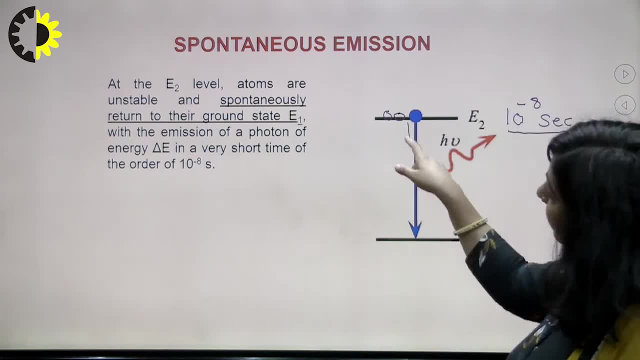 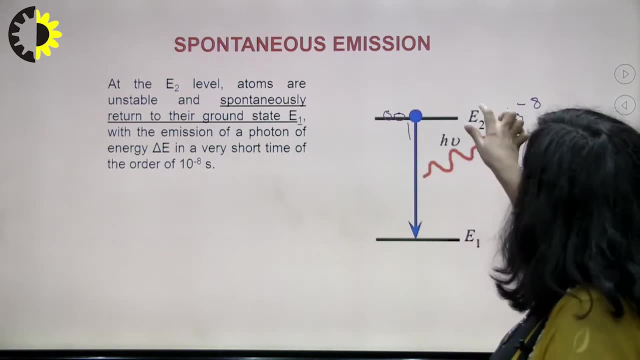 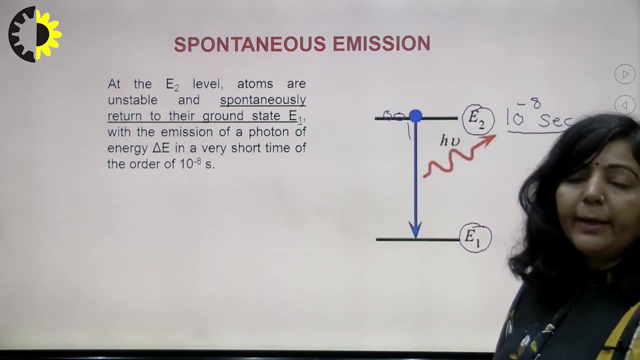 This state number 1.. And when they are coming down, They have to release their extra energy. Why they have to release their extra energy? Because In excited state They have energy E2.. And in ground state The energy of atom should be equal to E1.. 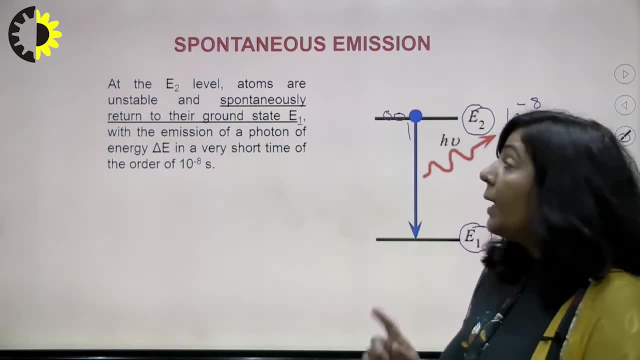 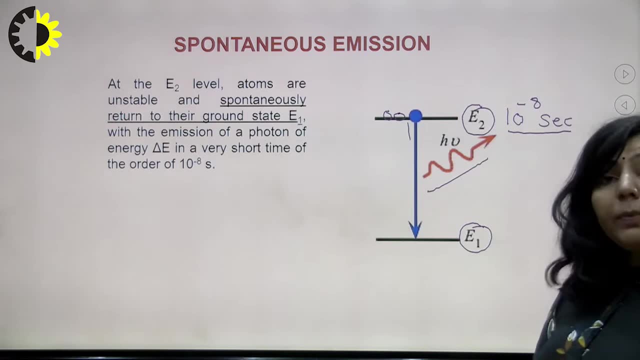 It means They have an excessive energy of E2. Minus E1.. So when these atoms are coming down, They will emit energy In the form of this photon. So this photon will be released And that photon is having energy. 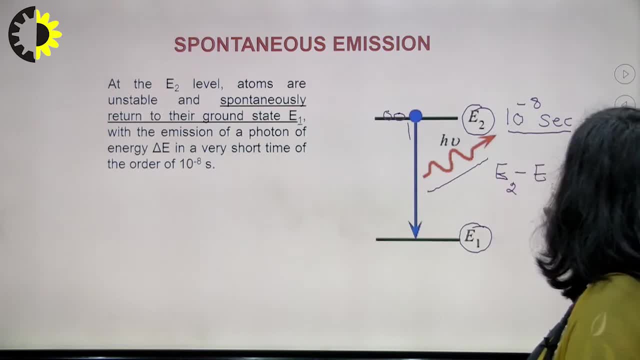 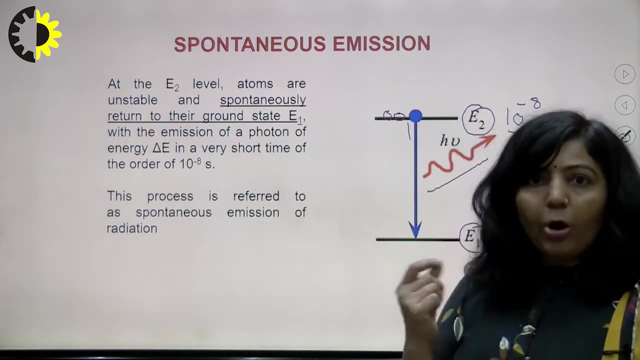 E2 minus E1.. So During this process, Since photons are emitted, So this process is known as emission process. And one more thing is there That, since You don't require any external trigger, here Means Automatically After completing this lifetime. 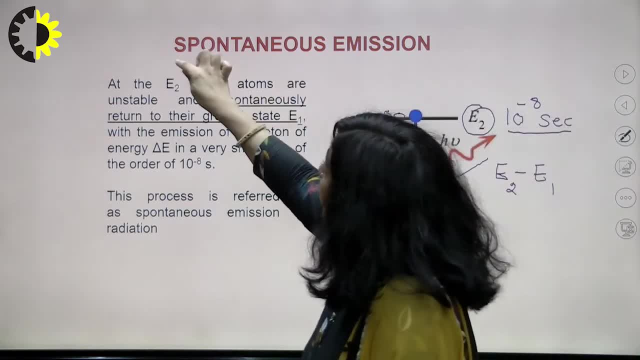 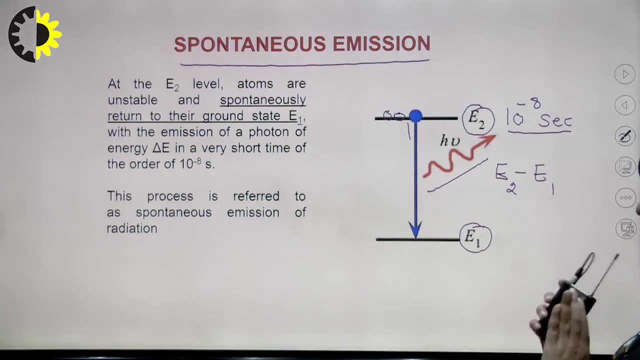 Atoms are coming down, So this emission process is A natural process. So that is the reason This is known as spontaneous emission. So this is the second process Which is involved in light amplification In case of laser. I hope this process is clear now. 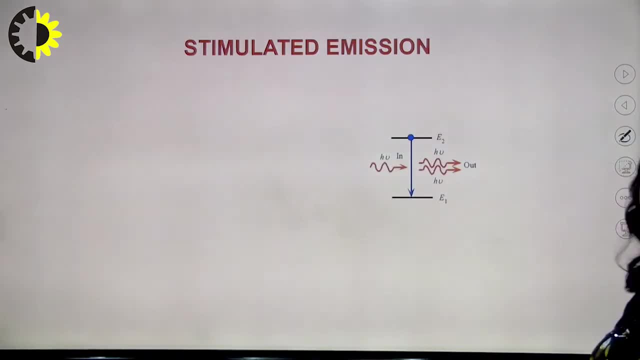 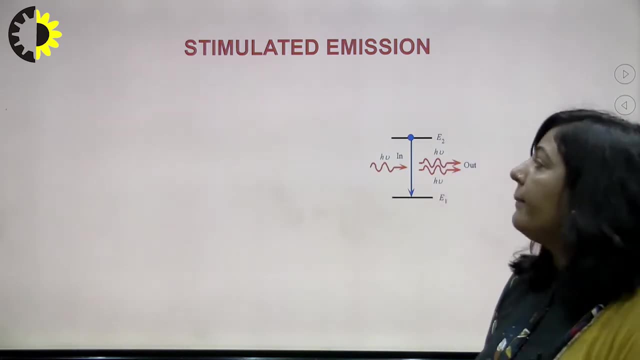 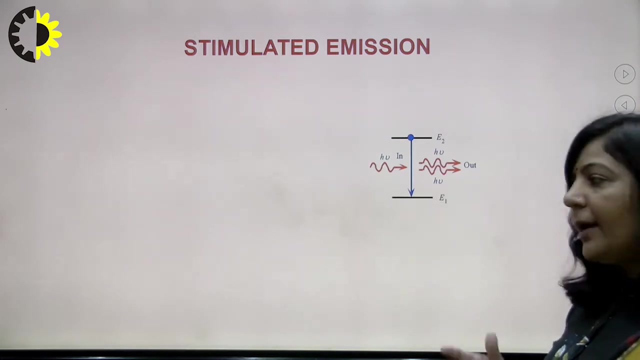 Now The third process, Which is the main process In case of amplification of light in laser. So that is stimulated emission. So in order to understand That stimulated emission, Again you have Same assembly of atoms, Again same situation is there. 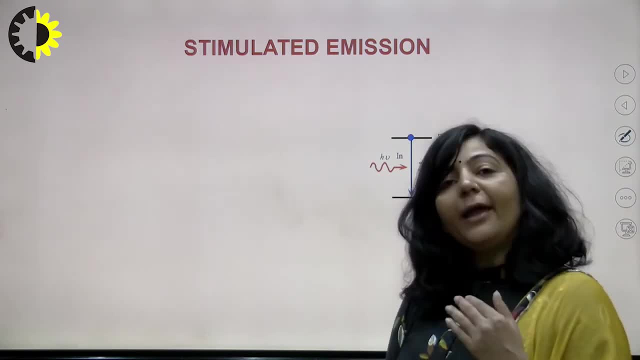 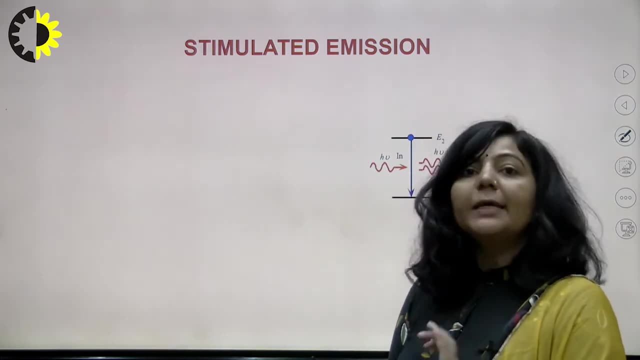 N1 atoms in ground state. N2 atoms in excited state, N1 or E1. That particular state is the ground state And N1 is very high as compared to N2.. Because state 1 is The ground state And more stable state. 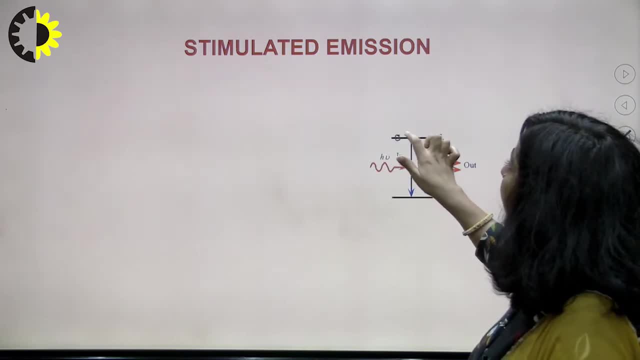 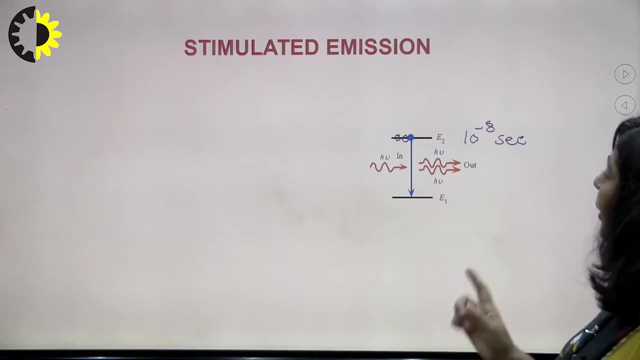 So, in this process, What you have here? Again, you have N2 atoms in this particular state, And you also know That the lifetime of these atoms Is 10 raise to power minus 8 seconds. Only for this duration Atoms can stay here. 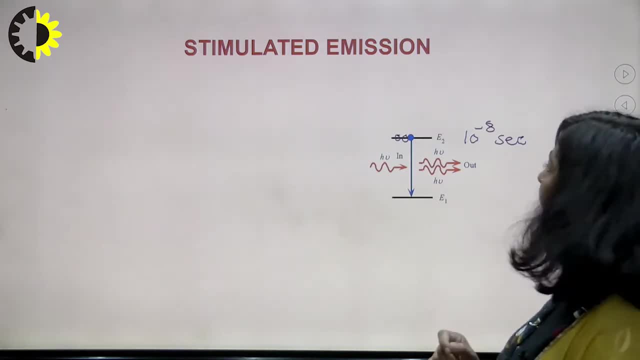 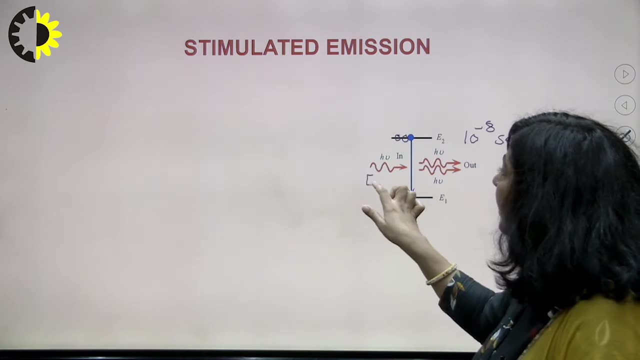 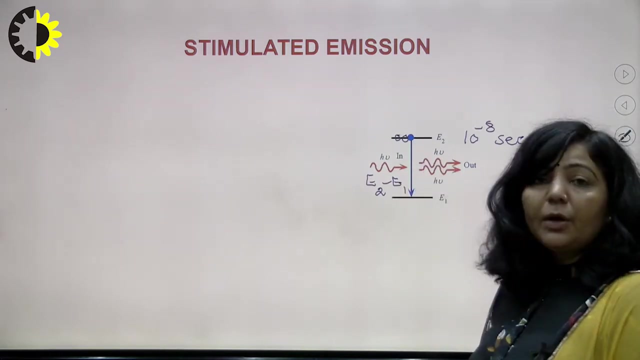 Now In stimulated emission, What we have? We have a photon here, And that photon Is of energy, And this photon Is interacting With excited atoms Before the completion of lifetime Of atoms in Excited state 2.. 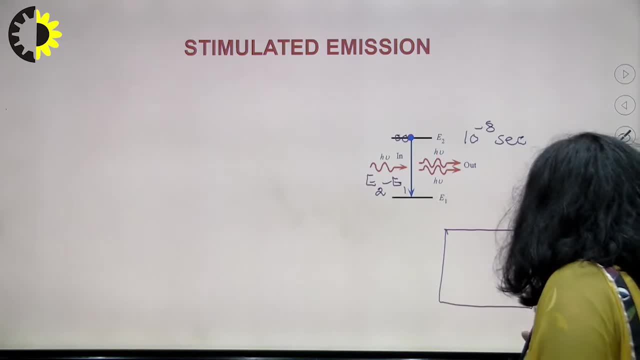 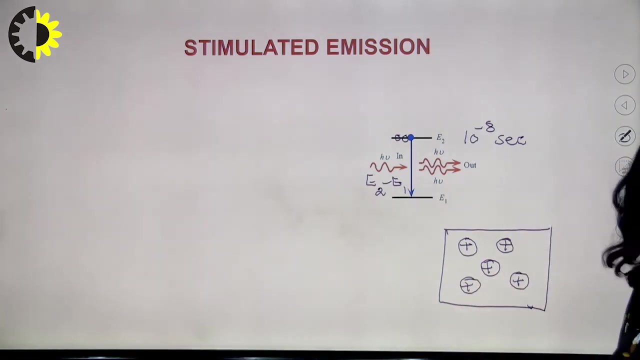 You can understand it like this: You have this assembly of atoms. In this assembly of atoms, Now, these, These are the atoms of Excited state. Suppose, these atoms, These circles with plus sign, Are the atoms of excited state With energy E2.. 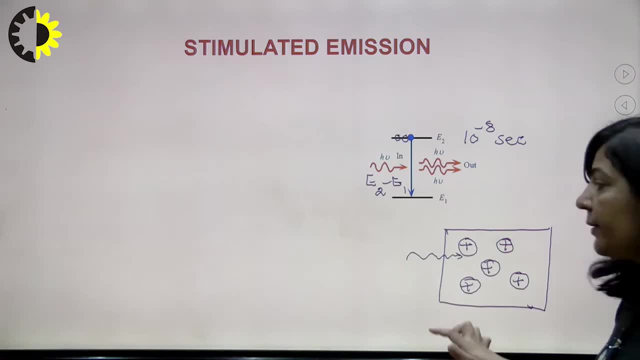 Now we are having a photon. This photon is coming And this photon is having energy: E2 minus E1.. Now this photon Is interacting With this excited atom. Now, this excited atom, It has not completed its lifetime In state number 2.. 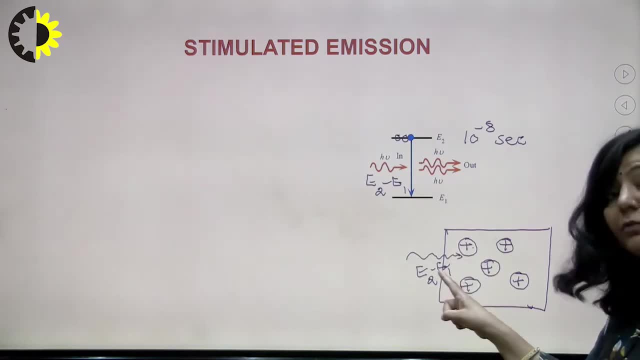 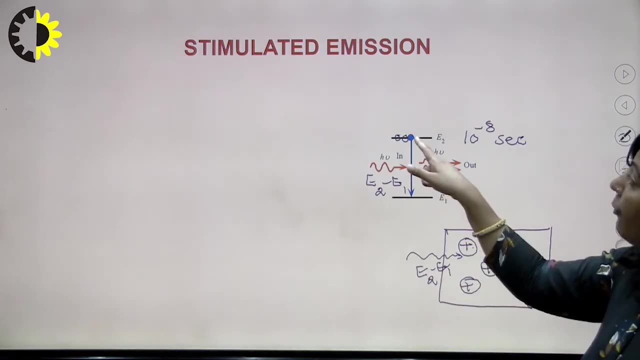 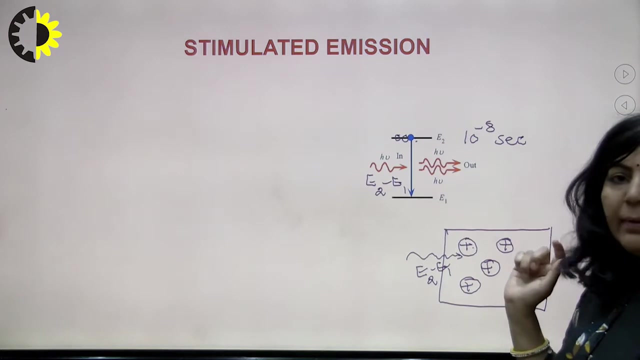 So, because of the interaction between these two, Because of interaction between the photon And excited atom, This photon Is forcefully sending Atom from excited state to Ground state, Means there is a transition From 2 to 1.. Before the completion of a lifetime: 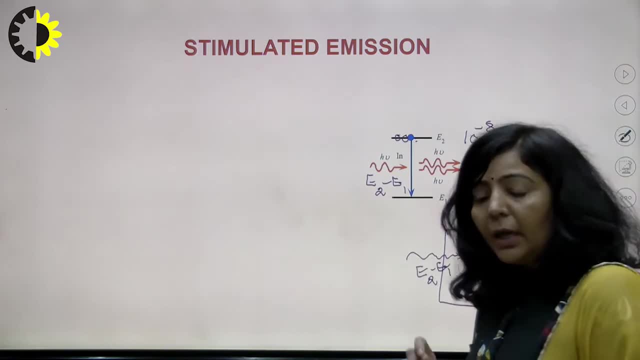 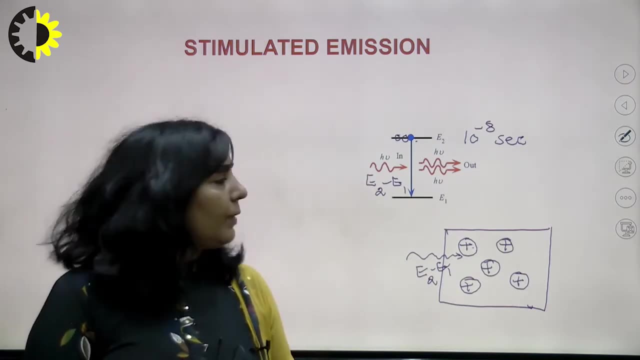 Of 10 raised to power minus 8 seconds. Because If the lifetime of 10 raised to power minus 8 seconds, If that will be completed, Then atom will automatically That will come down to 1. And that will be spontaneous process. 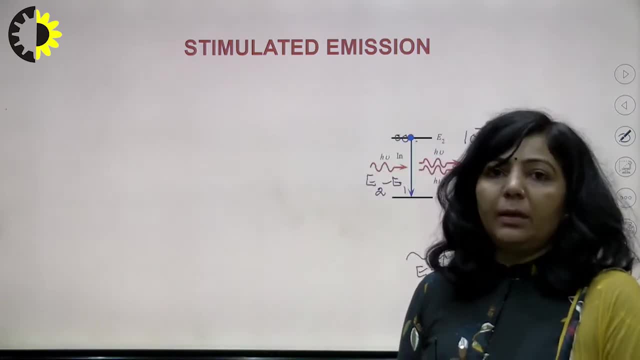 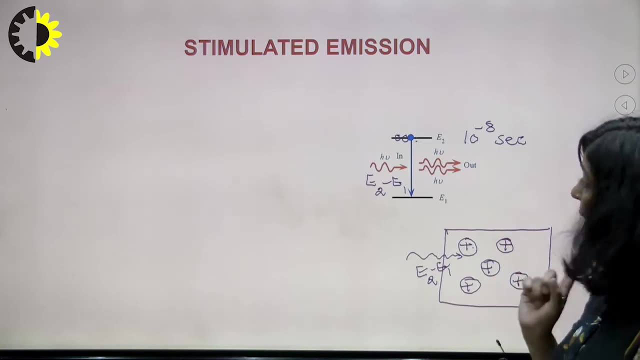 But here atom is not coming Spontaneously, Atom is stimulated, Atom is triggered for that transition From 2 to 1.. So this particular transition, When it will take place, From 2 to 1. You will get a photon of extra energy. 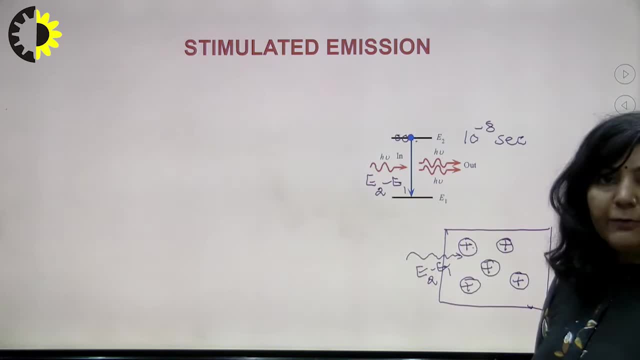 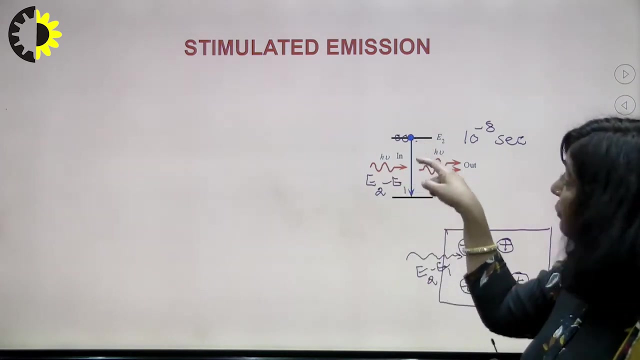 And that photon is Of energy: E2 minus E1.. So since The photon is emitted, So this is emission process, And since this transition From 2 to 1.. It requires a trigger, It requires a photon For the transition from 2 to 1.. 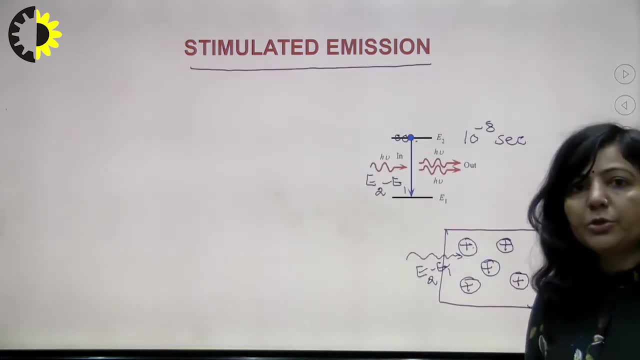 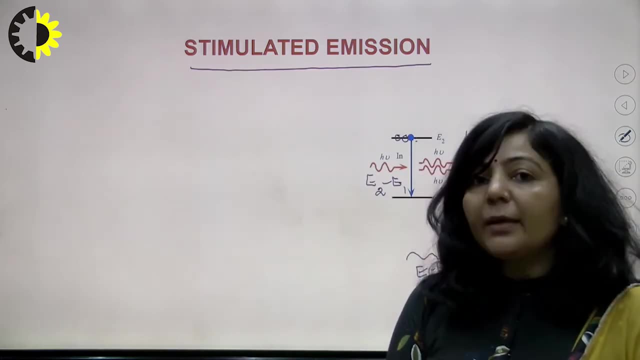 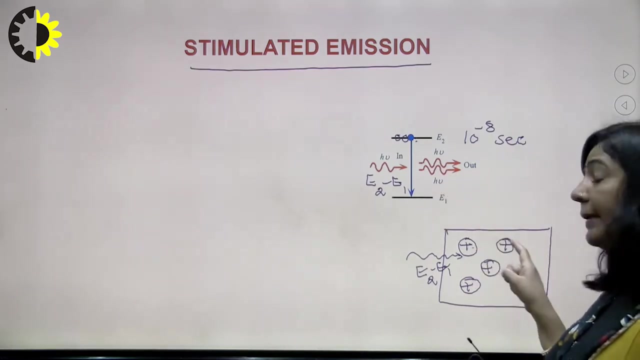 So that is the reason This process is known as stimulated emission process. So again, I am repeating This particular process Because you should understand The difference between spontaneous emission And stimulated emission. In stimulated emission, What we have? We have excited atoms. 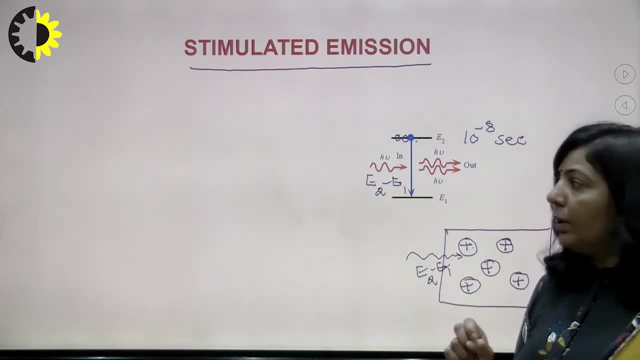 They are still in state number 2.. For a lifetime in state number 2.. Now a photon is coming, And that photon should have energy: E2 minus E1.. Now this photon of this much energy Is interacting with these excited atoms. 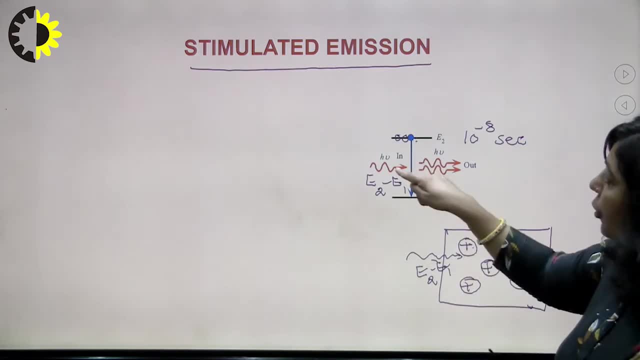 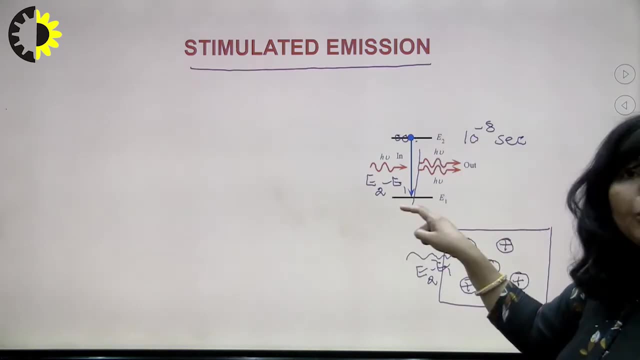 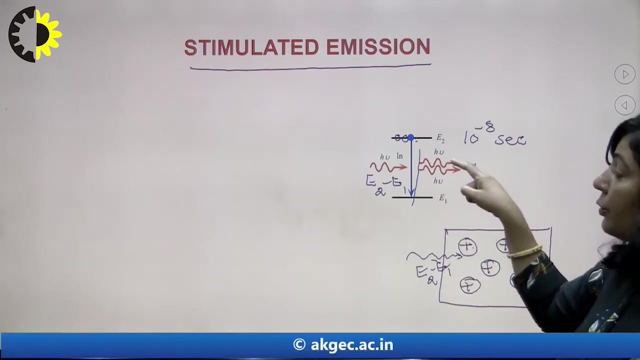 And because of that interaction Photon is forcefully Sending atom From 2 to 1.. So there is a forceful transition From state number 2 to 1.. And because of that transition Photons are, Photon is emitted. 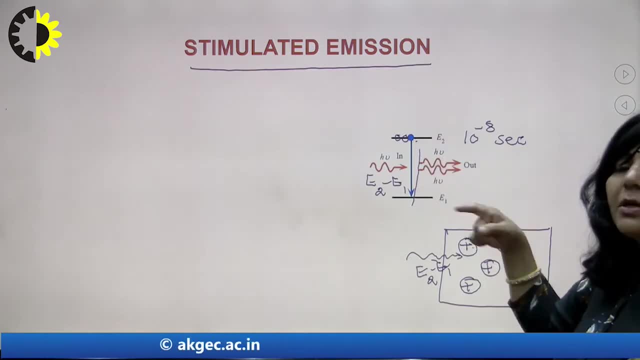 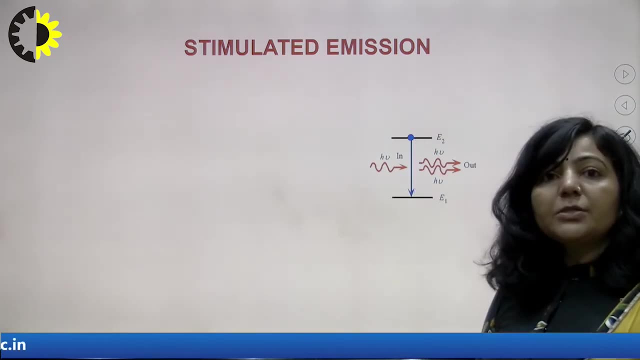 In stimulated emission process And since it is not a spontaneous process, So it is stimulated emission process. Now, the beauty of this process is Beauty of this particular process is That the photon Which is emitting this transition, This photon is responsible. 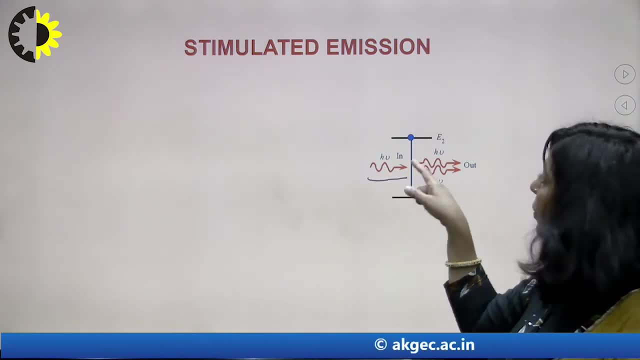 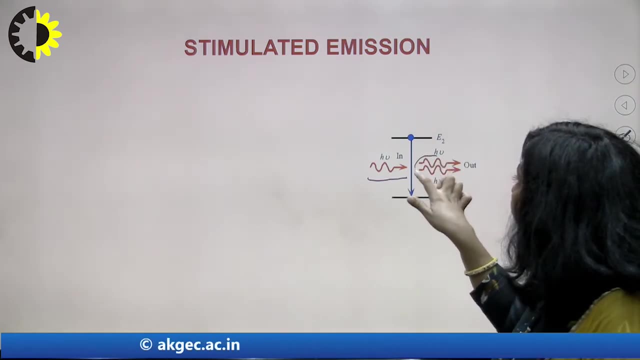 For stimulated emission. Because of this photon, There is a transition from 2 to 1. So you are getting another photon. So now, instead of 1. You have 2 photons here, And these 2 photons, As you can see here, 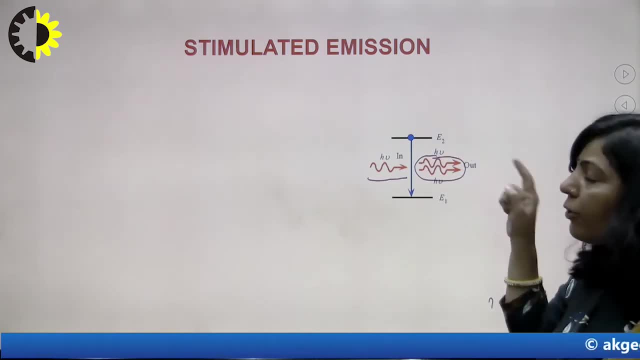 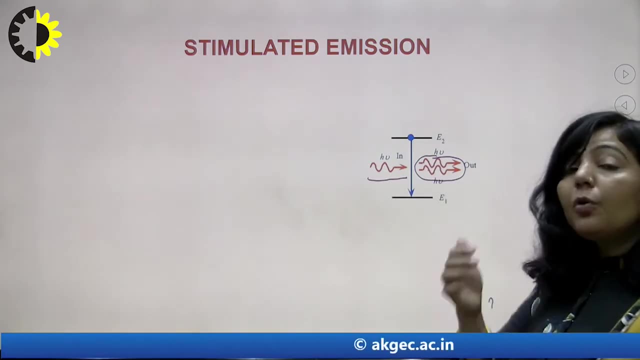 There is a crust to crust correspondence. Truffle to truffle correspondence Means these 2 photons. They are of same energy, They are in same phase. So 1 photon That is multiplied into 2. You are getting 2 coherent photons. 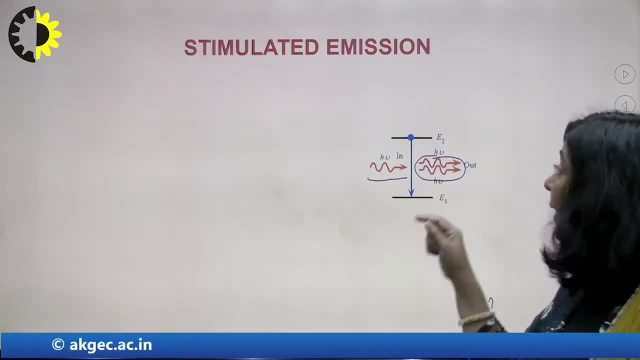 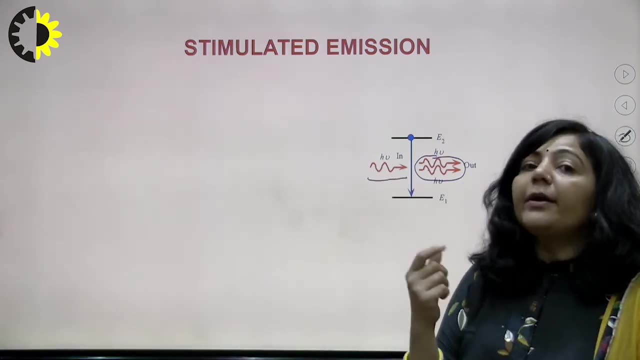 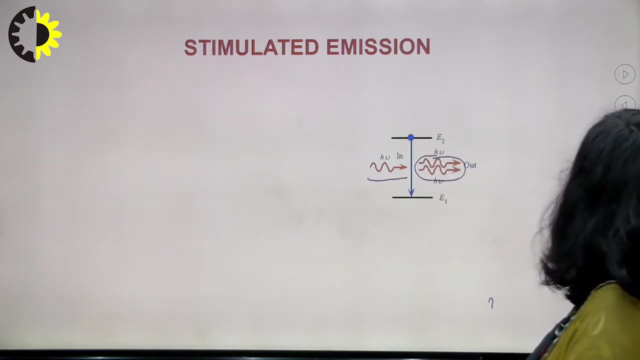 They are moving in same direction, They are having same energy And they are having a perfect phase relationship Between them. So 1 photon That is converted into 2.. Out of these 2. 1 is the incident photon And the other one is emitted due to 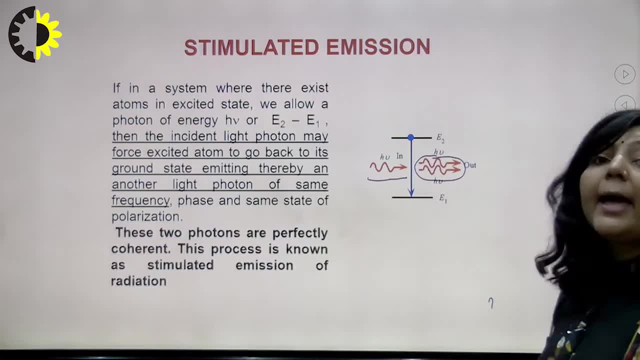 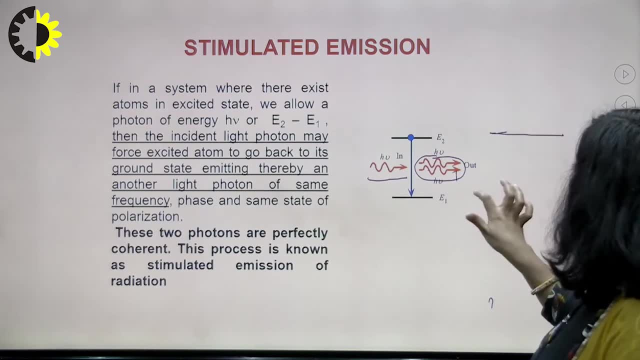 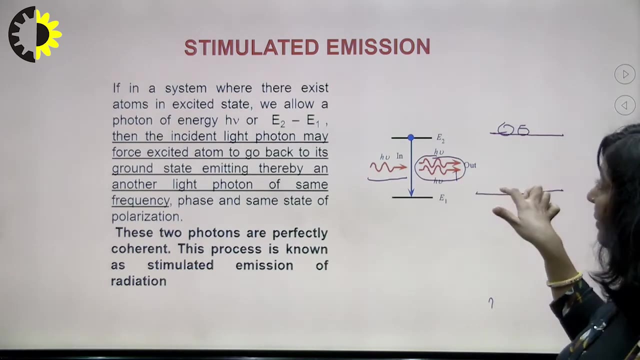 A transition from 2 to 1.. So this is your stimulated Emission transition. Now these 2 photons. You are getting 2 photons here. Now these 2 photons, They can interact With 2 more excited atoms. And if these 2 photons 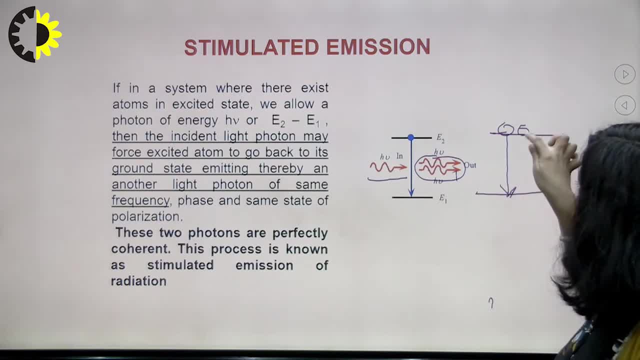 They are interacting with these 2 excited atoms, Then they can trigger 2 more downward transitions. So, finally, what you will get? You will get 4 photons. These 2 incident photons And 2 photons. They are emitted due to transition. 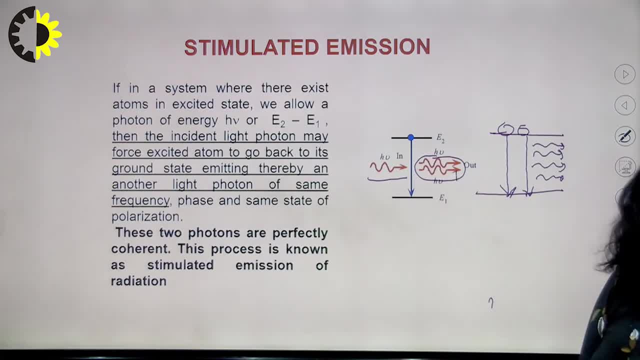 From 2 to 1. It means 1 photon is converted into 2. Then 2 photons, They will be converted into 4. And, as you can see here, All these photons, They are of same energy, All the photons. 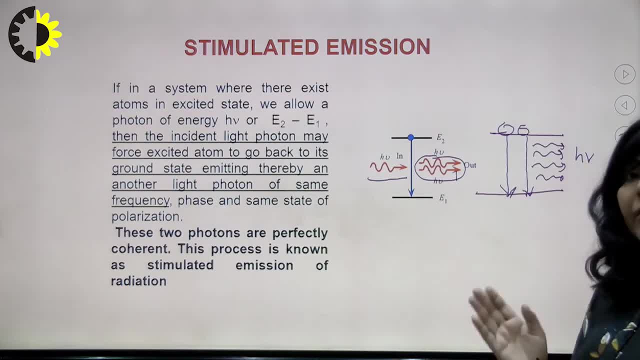 They are of same energy, They are in same direction And they are having a perfect phase relationship. So there is a multiplication of photons: 1 is converted into 2.. 2 is converted into 4. And this multiplication will go on. 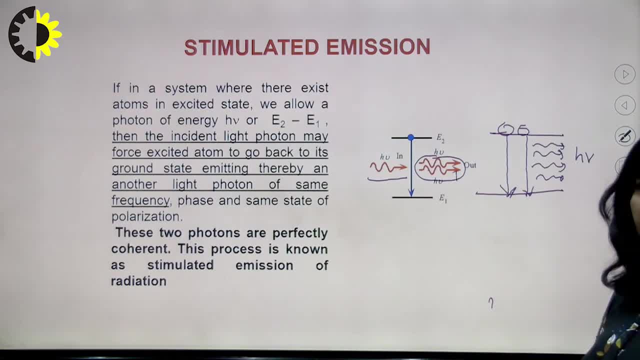 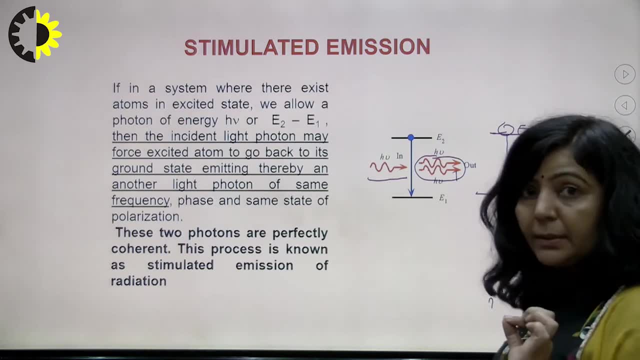 And then you will get an amplified laser beam. So this is the process Which is directly involved In light amplification In case of laser. So what we have discussed here, We have discussed our 3 processes, Which are the main processes in case of laser. 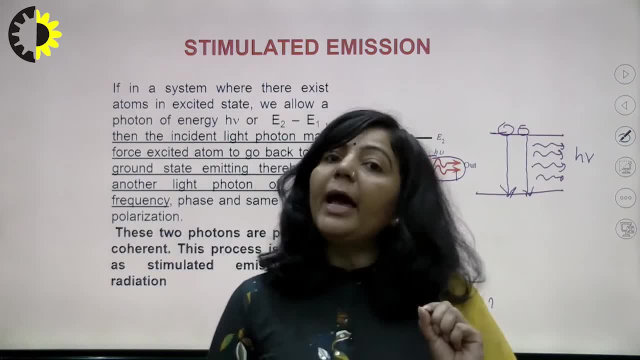 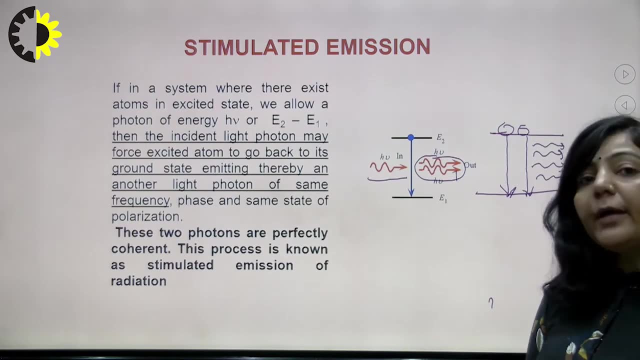 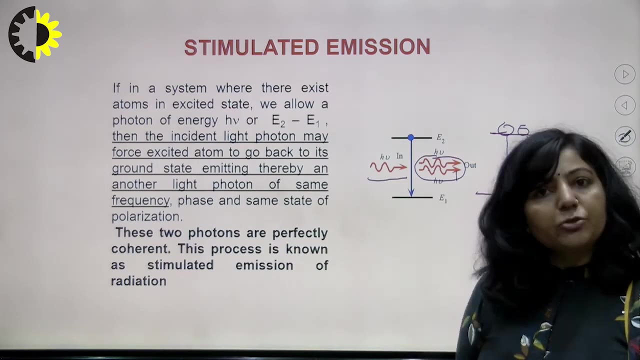 The first one is Absorption. Then we have spontaneous emission, Then we have stimulated emission. So absorption is always stimulated process, Whereas emission That can take place By 2 methods: Either spontaneous emission- That is, automatic- or natural process. 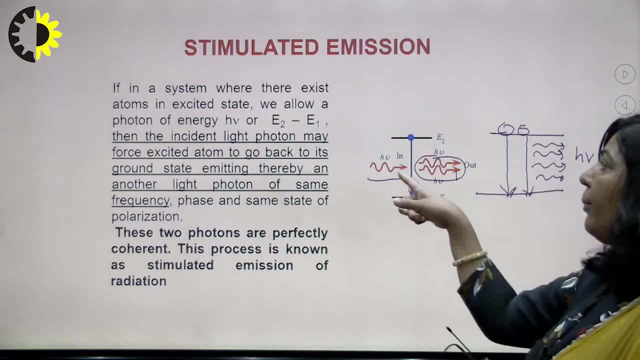 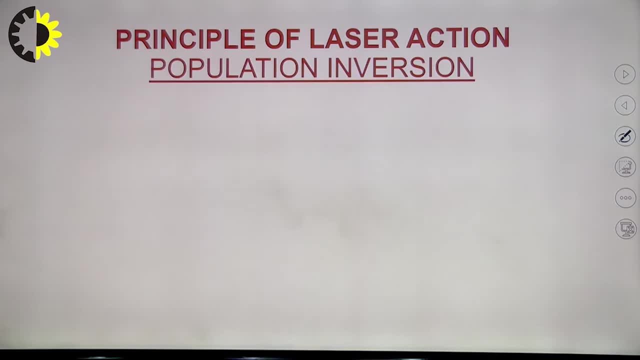 Or you have stimulated emission, And stimulated emission will take place With the help of this trigger. So these are the 3 processes. Now, the next topic Which I am going to discuss here Is the principle of laser action. That what is the basic idea. 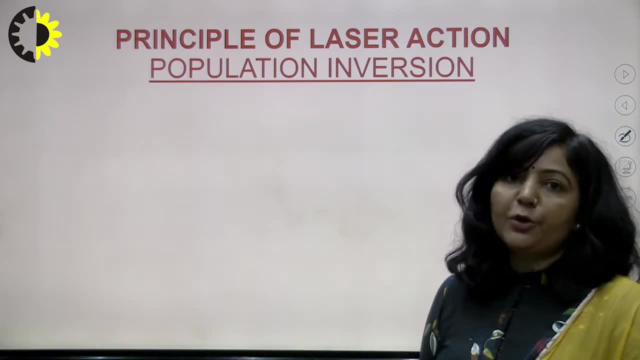 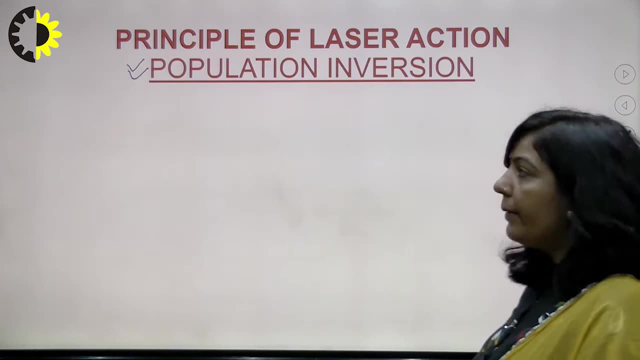 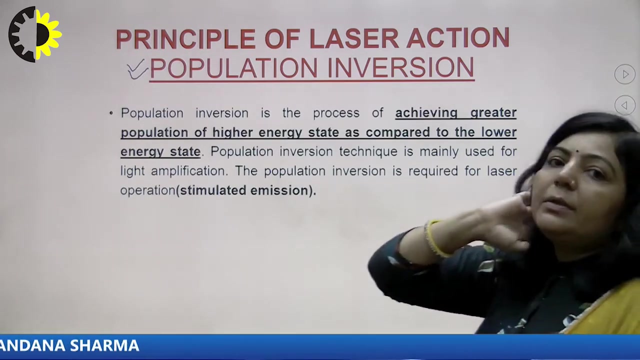 What is the basic principle Behind the amplification of light? And that principle is This one: Population inversion. Right, So now we will try to understand The meaning of this term: Population inversion. So population inversion means, Again, you have. 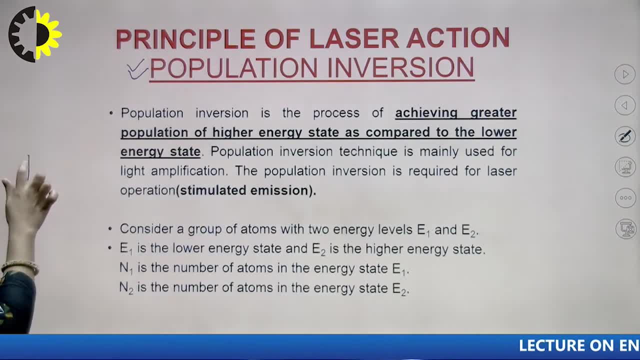 An assembly of atoms. You have an assembly Of atoms with NO atoms. And these NO atoms. They are distributed In 2 states: 1 and 2.. The population of state 1 is N1.. And the population of state 2 is N2.. 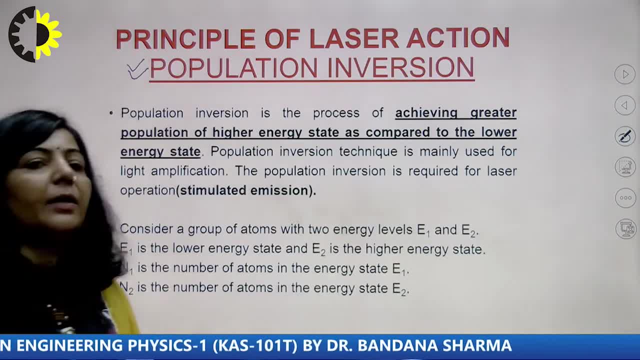 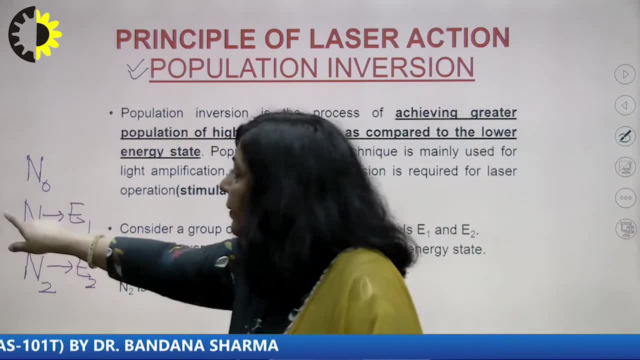 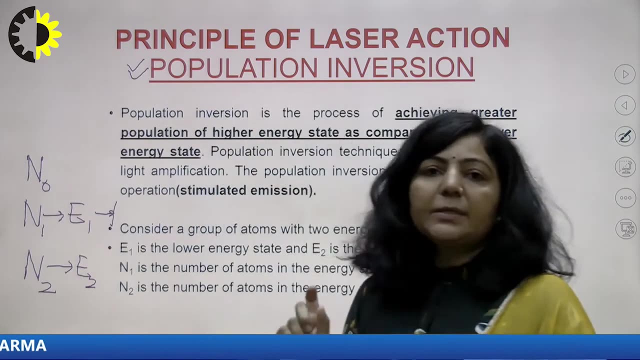 Energy of state 1 is E1. And the energy of Atoms of state 2 is E2.. Now, as I have discussed here That the state number 1.. This particular state, This state is Ground energy state And this particular state is having 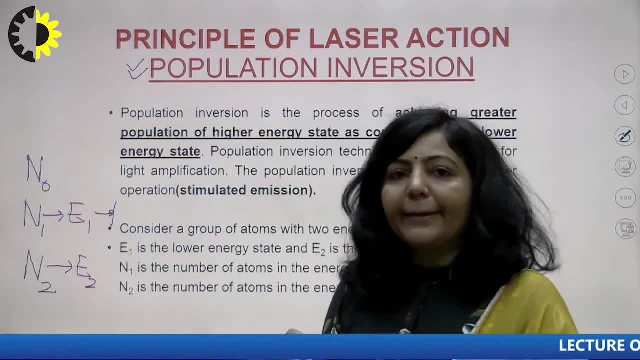 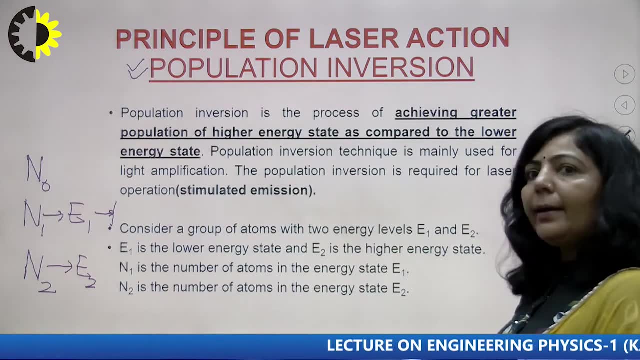 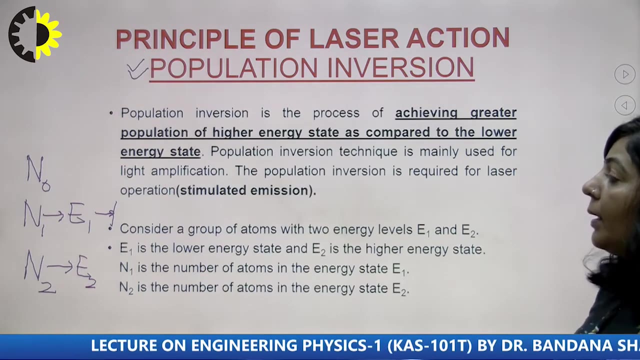 Most of the population of atoms, Or most of the atoms. They will try to remain in this particular state, State number 2. That is an excited state, Highly unstable state Because its lifetime is very small. So only few atoms Can exist in that particular state. 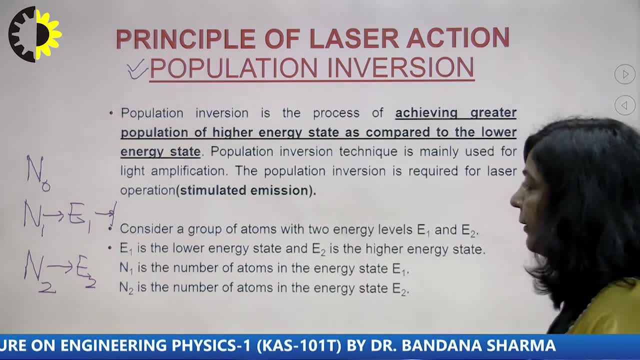 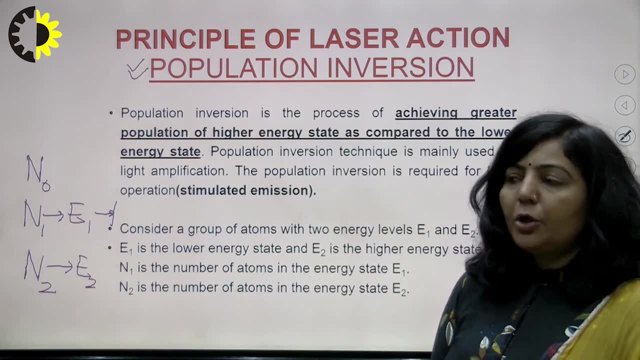 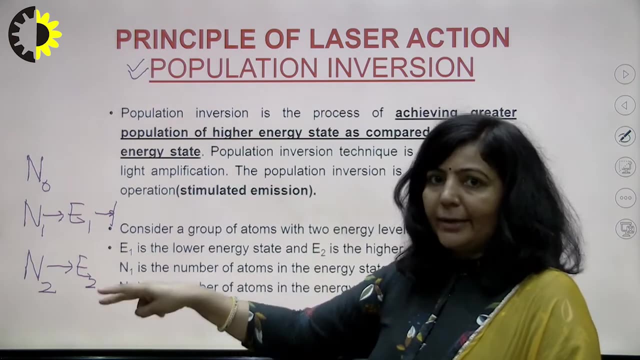 So what is the meaning of Population inversion here? So if you want to understand Population inversion, What is normal population of atoms? So from here You can say: If there are only 2 states, 1 and 2. 1 is the ground state. 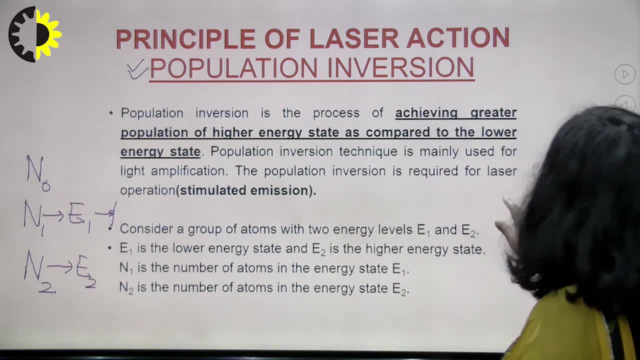 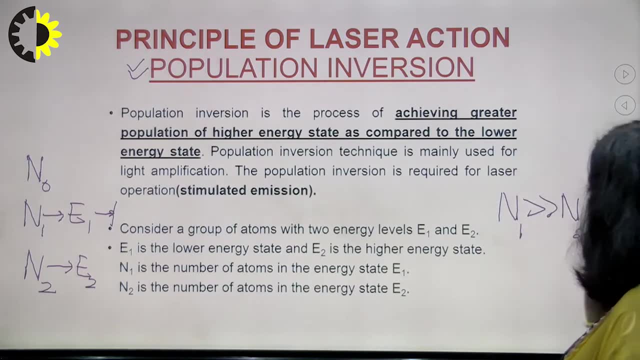 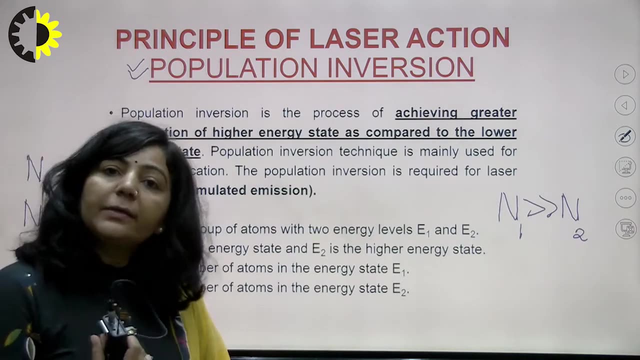 2 is the excited state. Then what will be the normal population? The normal population will be this N1 will be much, much greater than N2.. Is it right? You have to think on this State, number 1.. That is the ground state. 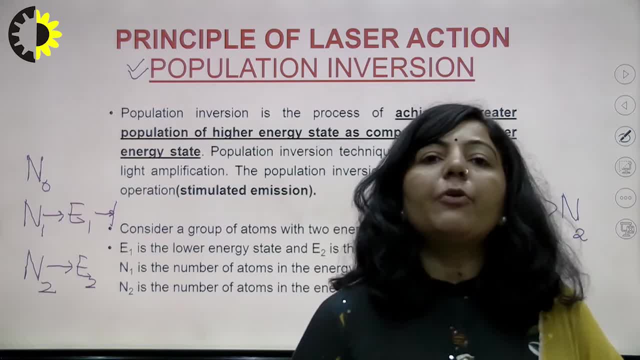 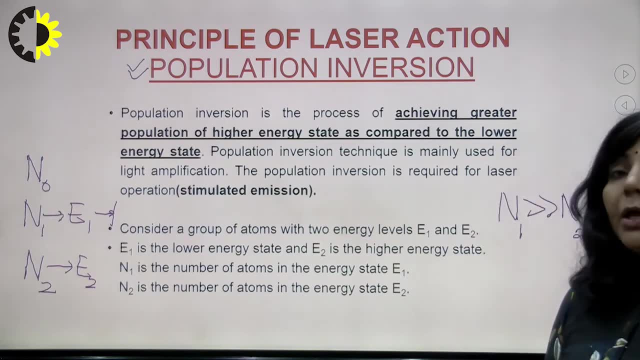 Most stable state. Most of the atoms They will try to remain in that particular state. State 2 is an excited state And only few atoms will exist in that particular state. So in normal conditions You can say The relationship Between the population of those 2 states. 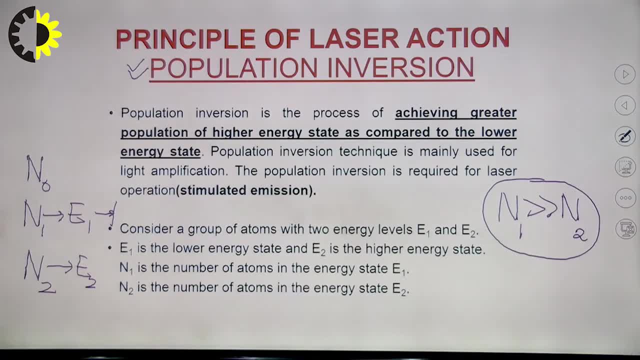 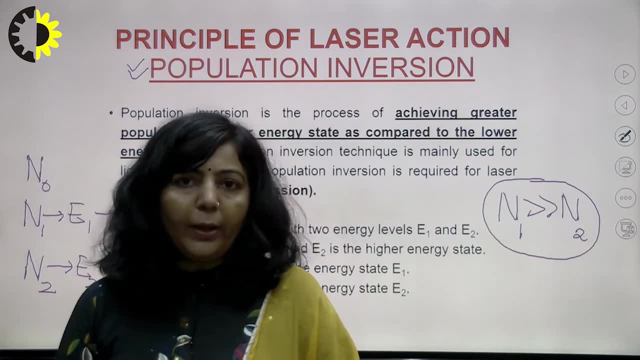 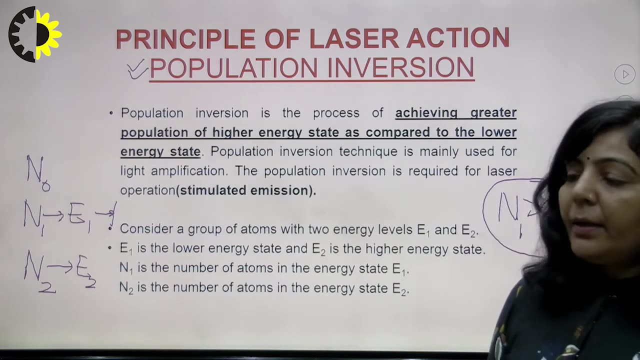 Is this? N1 is much, much greater than N2.. Now the next question is: If this is the normal population, What will be the probability of Stimulated emission? So you also know, Laser means light amplification By stimulated emission. 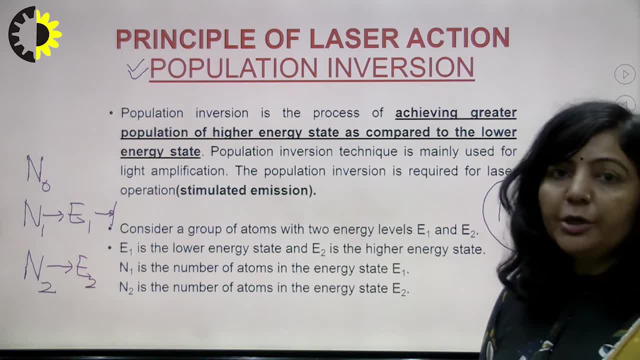 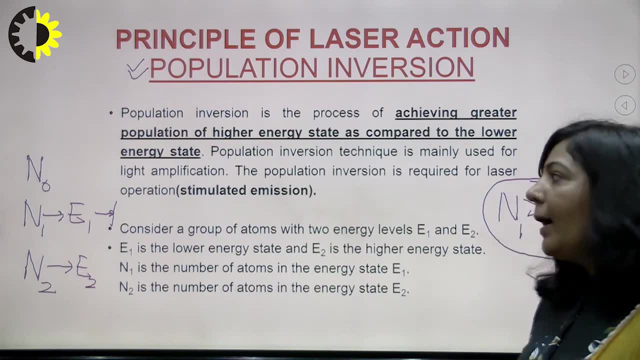 It means The probability of stimulated emission That should be very high. In order to get laser action, In order to get laser light, Stimulated emission, The probability of stimulated emission Should be very, very high. And you know That stimulated emission. 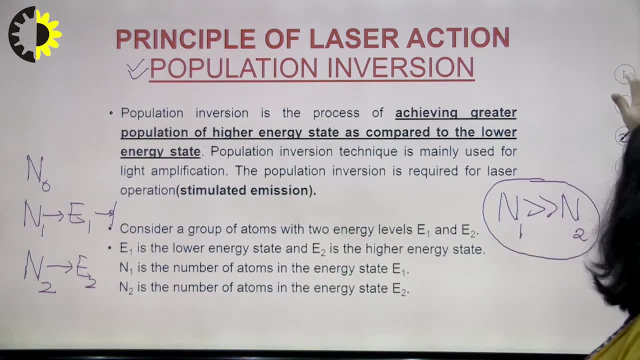 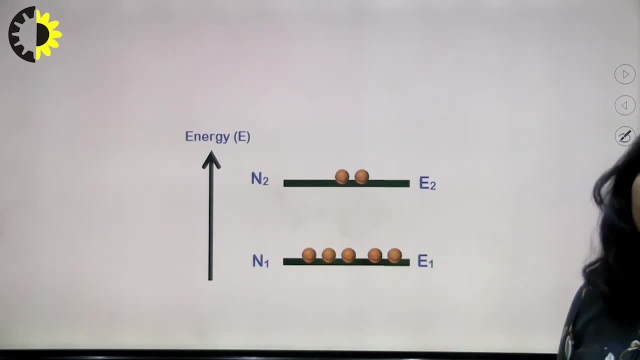 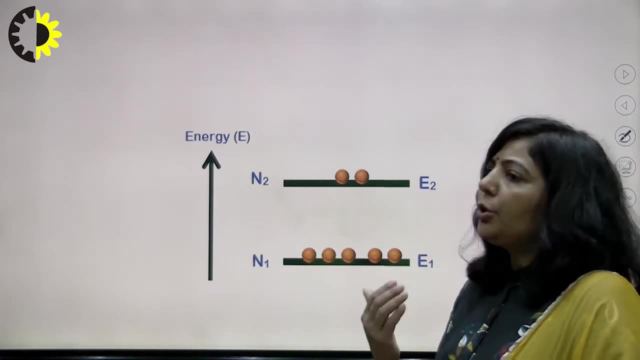 Is in excited state. If you have large number of atoms In excited state Only, then there is a possibility Of transition of those atoms From excited to ground state. So for stimulated emission, In order to increase the probability Of that particular process. 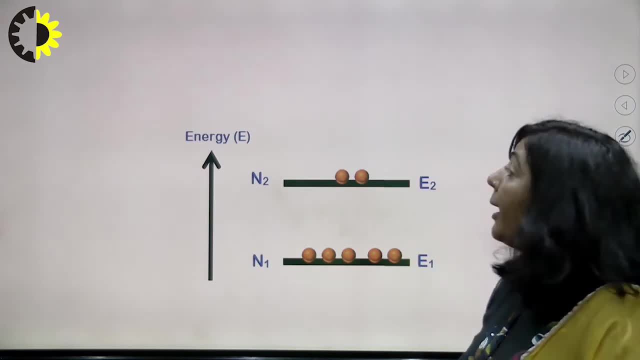 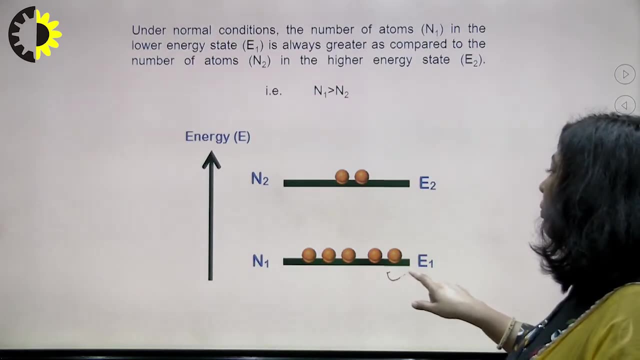 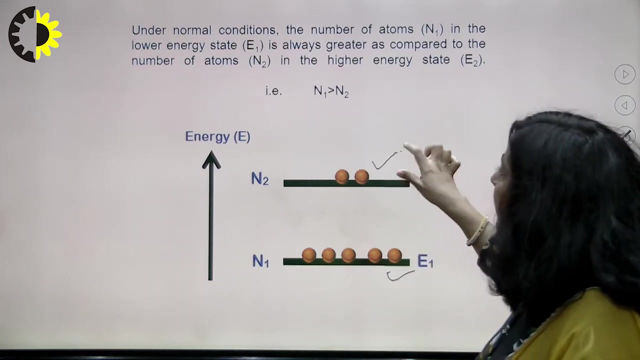 You should have a greater population Of atoms in excited state. But the problem is In normal conditions. This is the normal condition. In normal conditions It tries to remain in this Ground state or stable state, And only few atoms will be there. 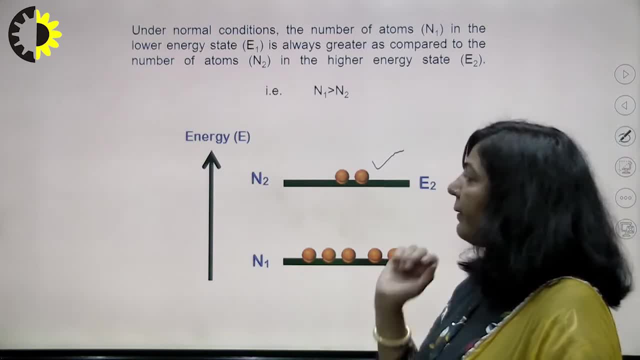 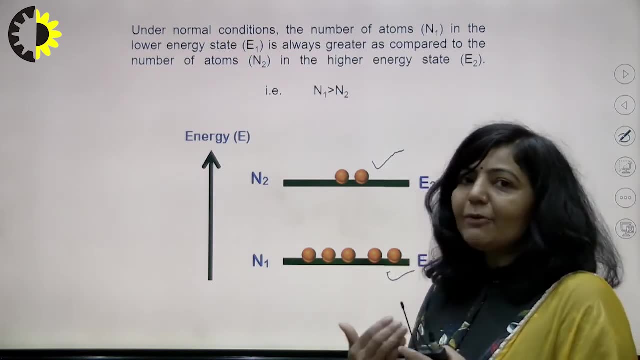 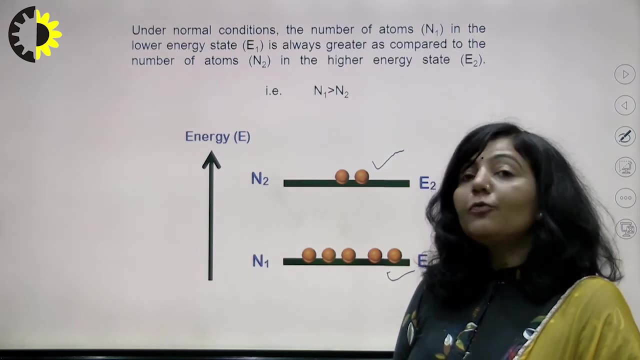 In excited state. So if you have only few atoms here, Then the probability of stimulated emission Is also very low. It means There cannot be sufficient multiplication of photons. It means You cannot get an amplified laser beam there. So what you have to do 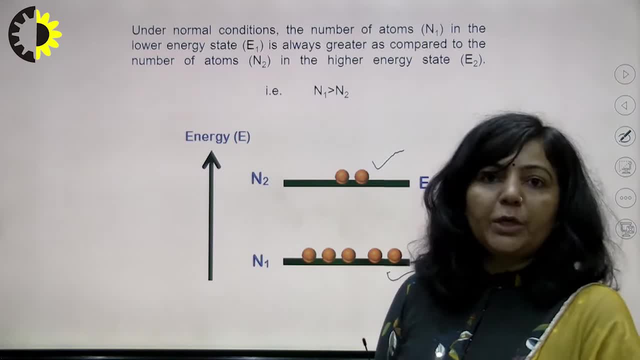 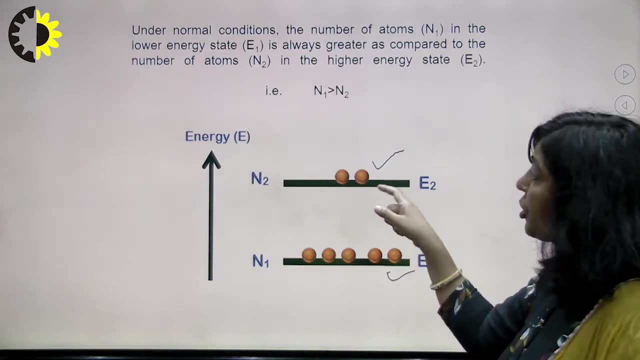 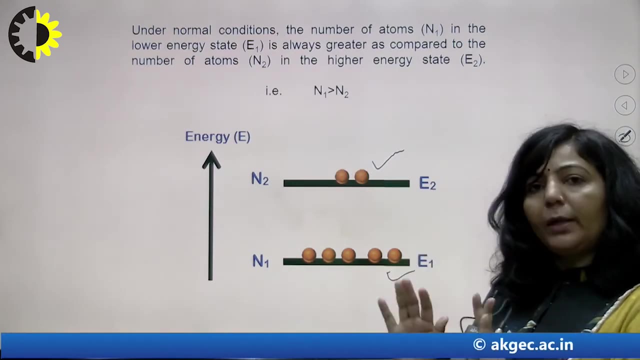 You have to Invert this situation. You have to invert this population Means We should have A greater population of atoms in excited state As compared to Ground state. The total population will remain same. Total atoms will remain and not 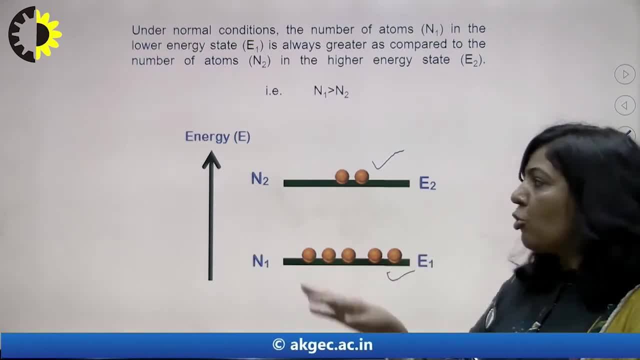 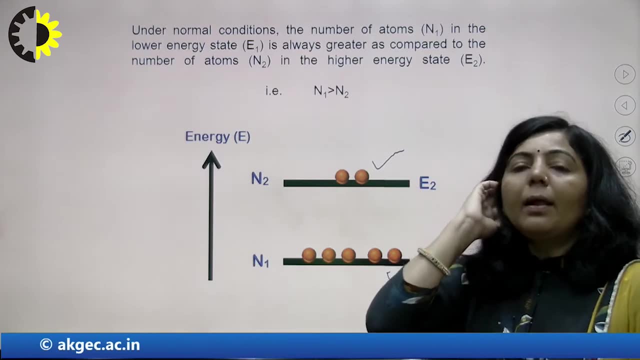 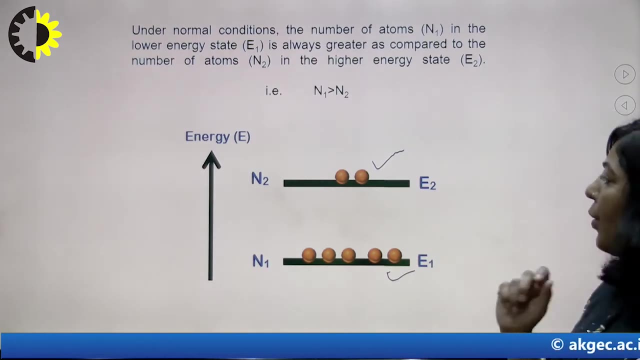 There can be redistribution of those atoms Between these two, In normal conditions, at a fixed temperature. This is the normal population. But you know, In order to get laser light You have to invert this situation, So That particular situation When you have more atoms. 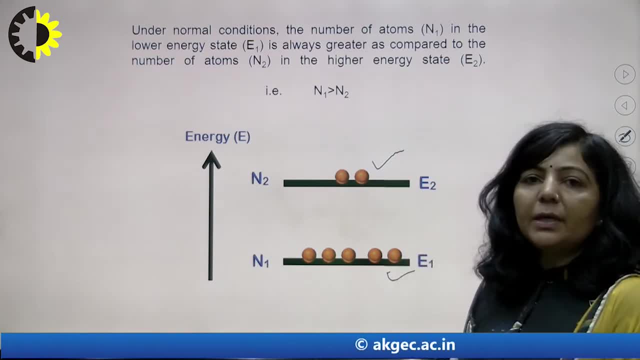 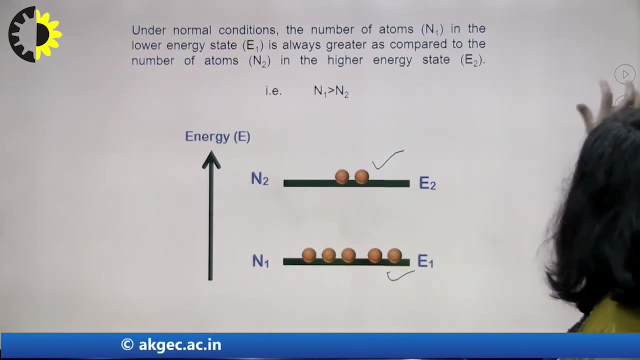 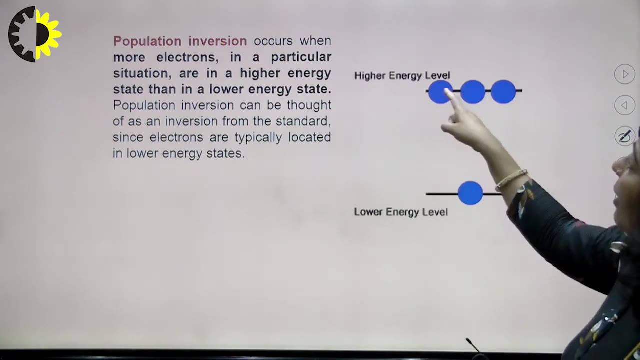 In excited state As compared to ground state. That situation, That state, is known as Population inversion state. So when you have, This is your population inversion state. When you have more atoms In excited state, Or high energy state, As compared to ground state, 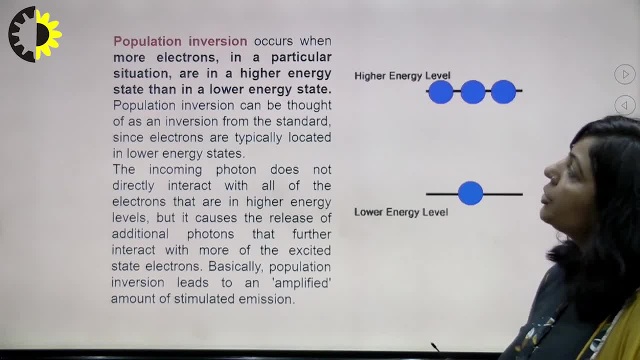 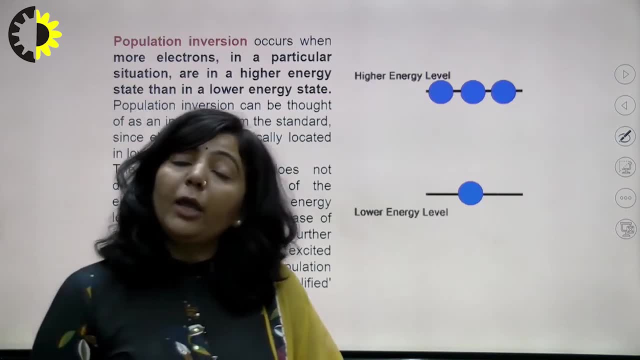 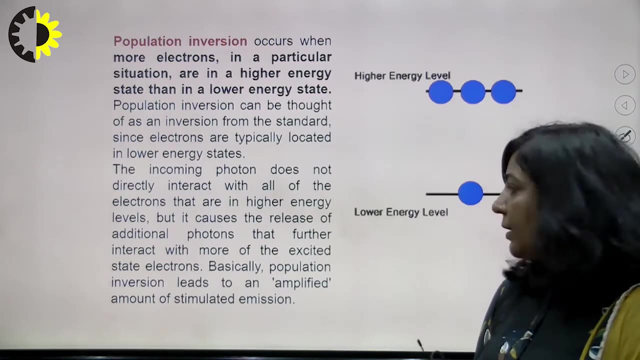 Then that particular state is known as Population inversion state. So You will get laser beam, You will get multiplication of photons Only if you can achieve this particular state Means Somehow you have to Pump those ground state atoms, You have to invert the population. 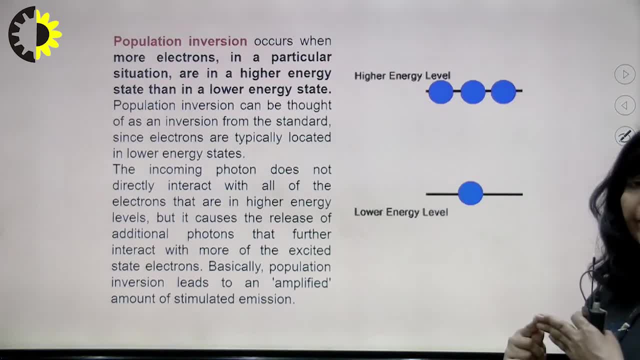 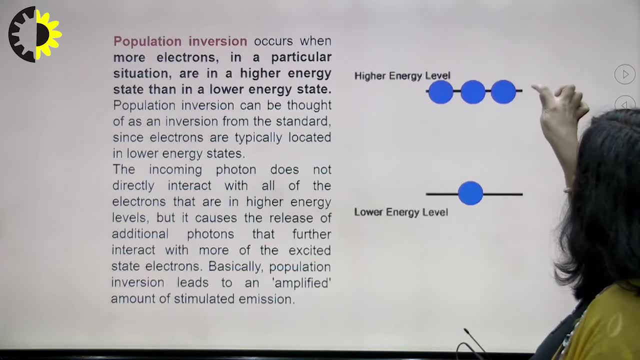 Means from one. You have to send atoms to excited state And you have to achieve that particular state When you have Population of atoms in Excited state: 2. As compared to ground state 1.. So when you are achieving this state, 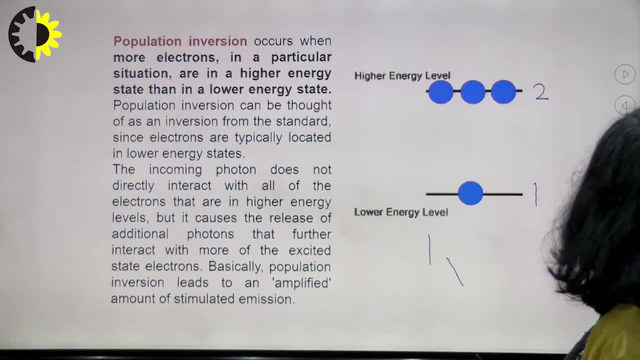 When you have N2.. Sorry, When you have this, Just give me one minute- When you have N2 greater than N1. Only after that You can think about Amplification of light. So it means The principle of laser action. 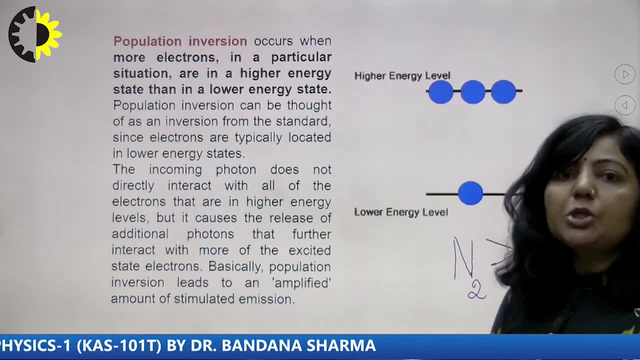 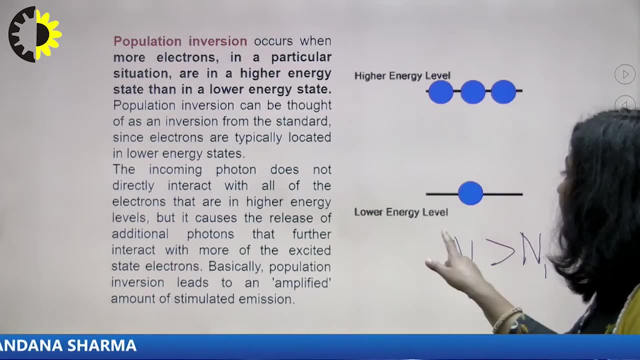 Or the main point. Think about the multiplication of photons, Or that particular point Beyond which you can think that There can be amplification of light. So this is the condition After which the amplification of light can take place. Means: 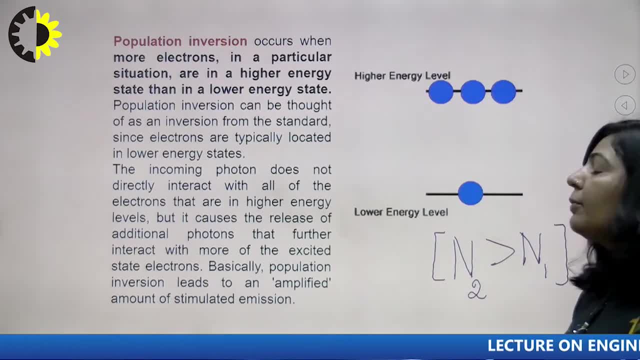 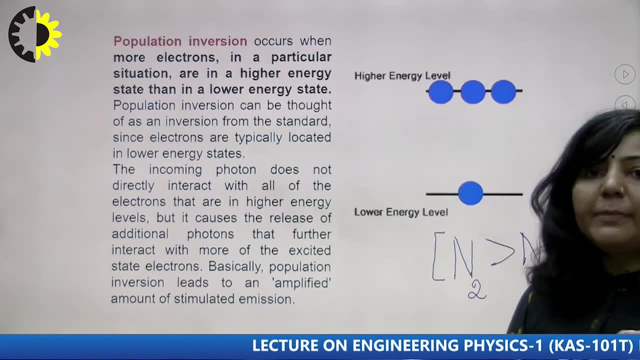 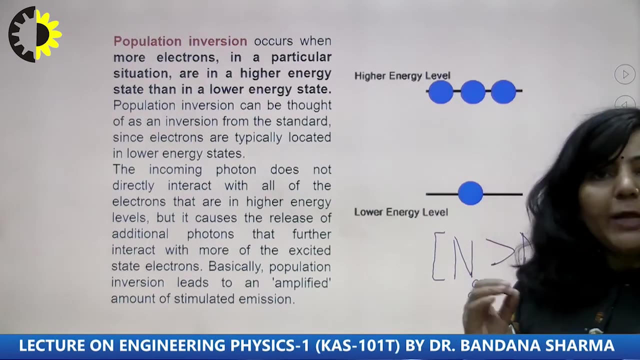 You have to exceed the population of high energy state As compared to ground state. So that is your population inversion. So I am summarizing Population inversion here. Population inversion means In normal conditions Most of the atoms Are in ground state. 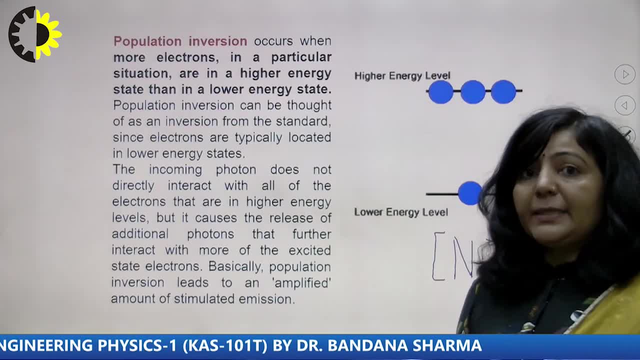 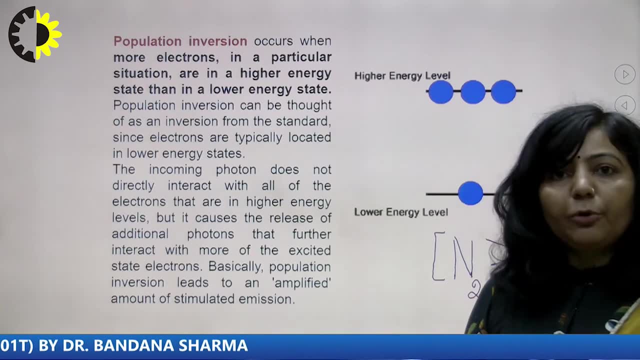 So that is a normal population. But in order to get laser light, In order to get Amplification of light, We have to achieve that Stimulated emission process, We have to increase the probability of stimulated emission And the probability of stimulated emission. 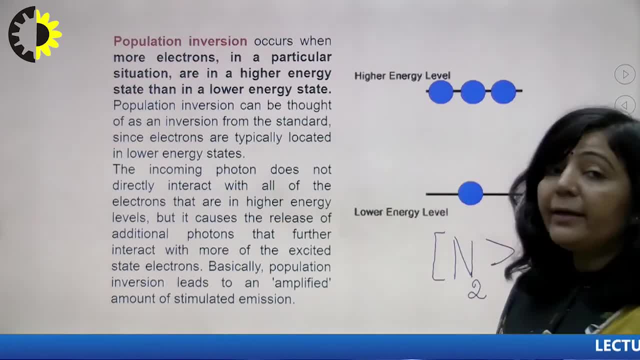 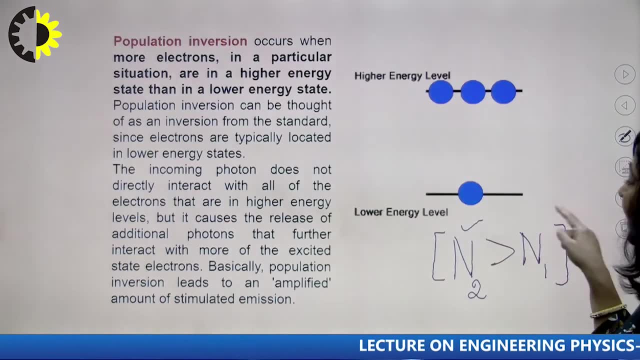 That depends upon The population of high energy state. It means somehow We have to invert the population. So when you have more atoms In excited state, That state is known as Your population inversion state. So this is the principle of 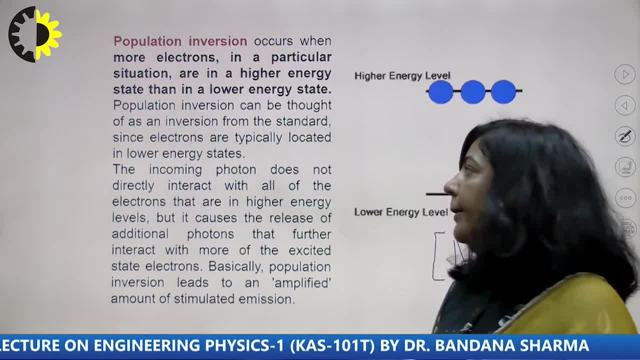 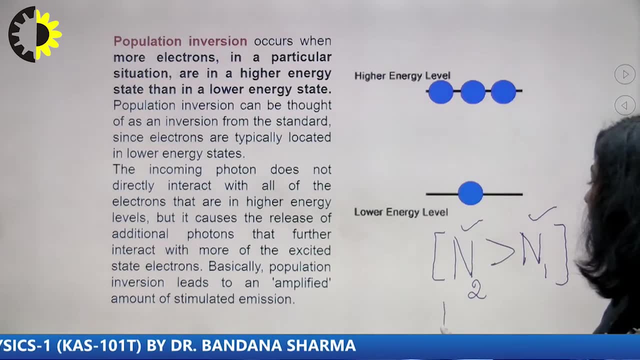 Laser action. And one more point: you have to remember here: The process, The method Through which you will achieve this population inversion. This is population inversion, So the process through which you will achieve this population inversion. That process is known as: 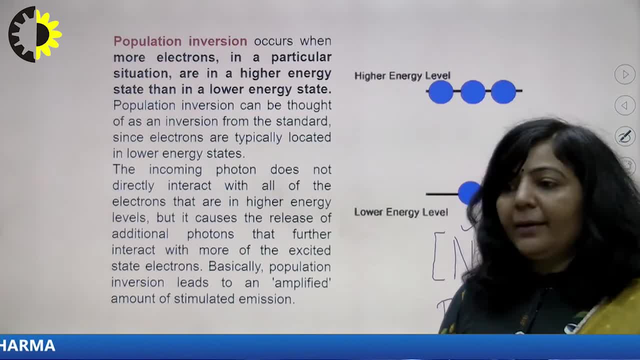 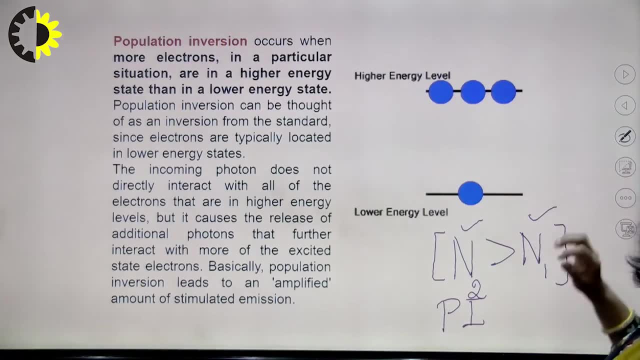 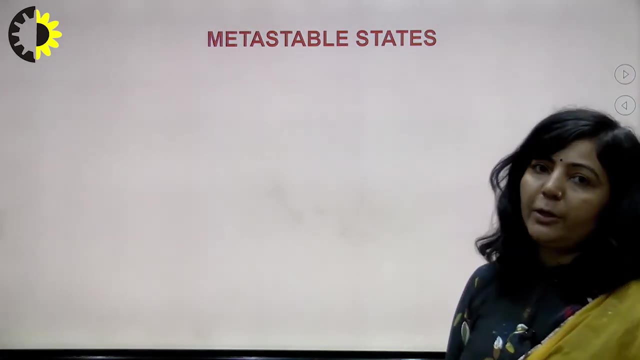 Pumping process Or pumping method, And we will discuss this pumping method In detail In the next class of laser system. So this is your Principle of laser action. Now, the next topic Which I am going to discuss here is: 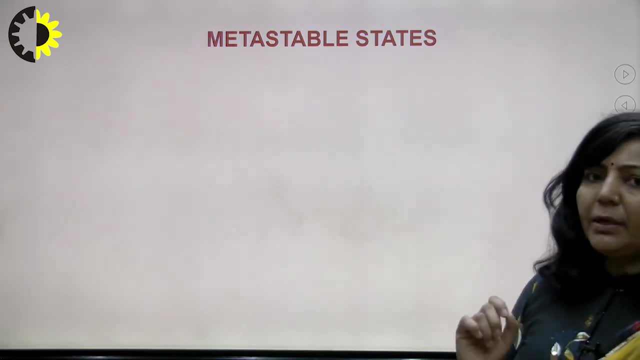 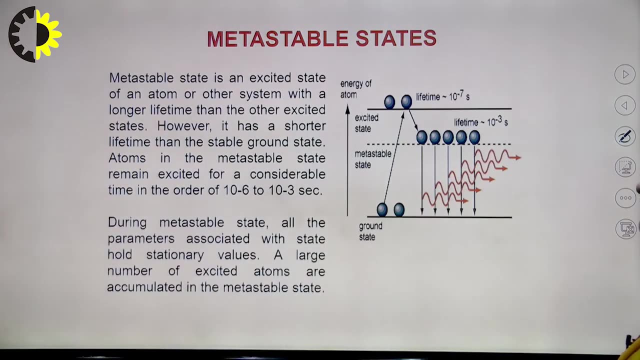 Metastable states. So, metastable states, These states are very important, Very essential In order to get amplification of light In case of laser. So in order to understand that What we are taking here, Again, we are taking only two states here- 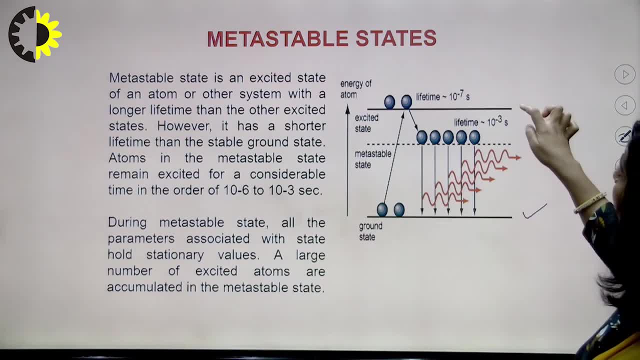 State number one: This is your ground state. State number two: This is your excited state And a very short lived state With a very small lifetime of approximately 10 raise to power minus 7.. 10 raise to power minus 8 seconds. 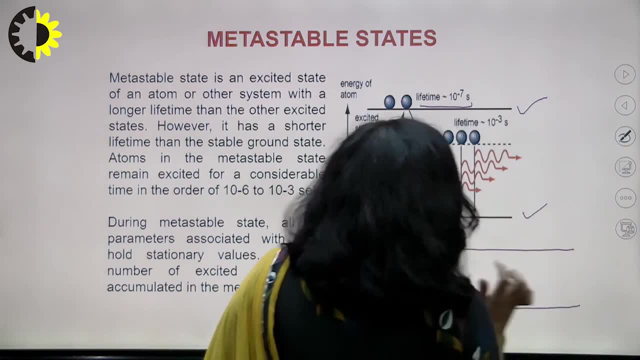 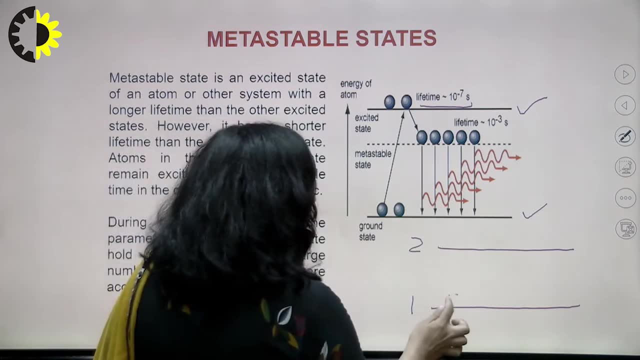 If you have only these two states, Suppose in your assembly of atoms You have only these two states, That is, one and two. If you have only those two states, Then you know, in normal conditions Most of the atoms Will be there in ground state. 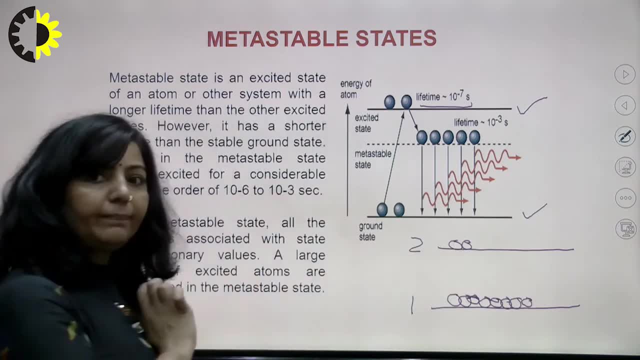 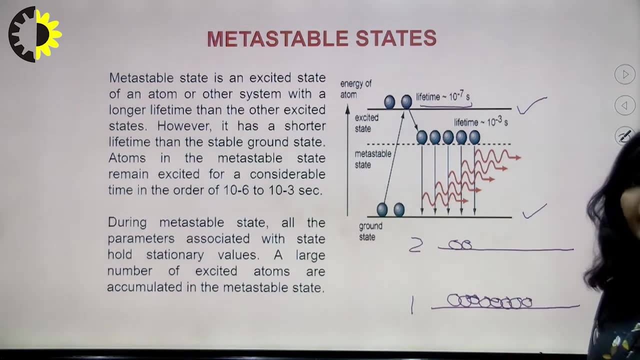 And only few atoms will be there in Excited state And, as you have discussed here That you have to invert the population, You have to exceed the population of atoms in Excited state As compared to ground state. You have to achieve population version. 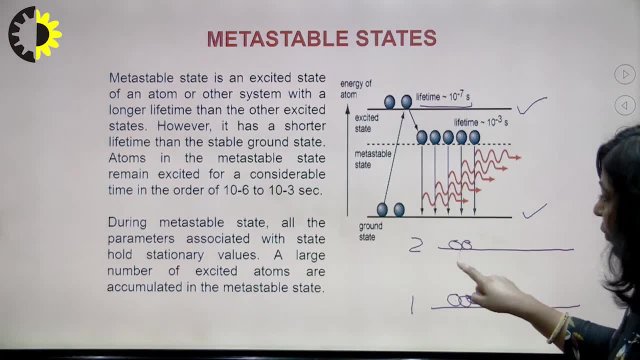 Now suppose You are sending these atoms from one to two. These atoms are pumped With the help of an external energy source. These atoms are pumped from One to two. If these atoms are going from one to two, Then The population of this state? 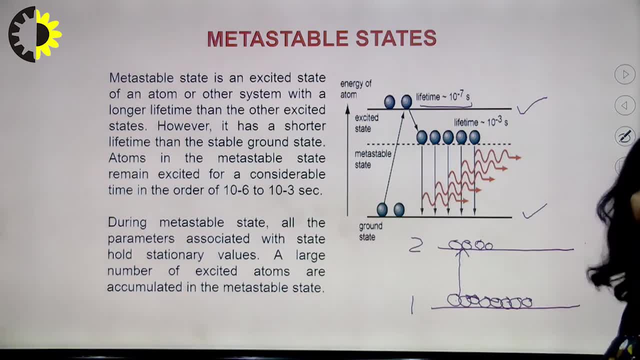 State number two will start increasing. But the problem is The atoms. They cannot stay here for a longer duration. They will stay here Only for this small duration: 10 raise to power minus 8 seconds. Now what you are doing. 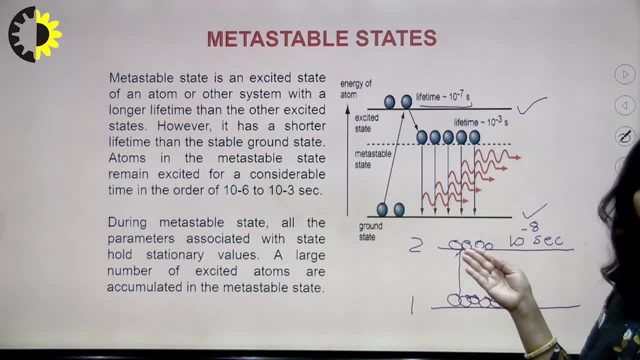 You are pumping these atoms from one to two, But in two They are not staying for a longer duration, They are automatically coming down to one. It means You can never achieve a state Where n2 is greater than n1.. It means 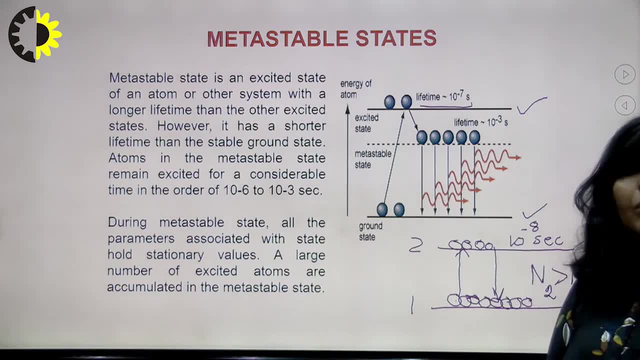 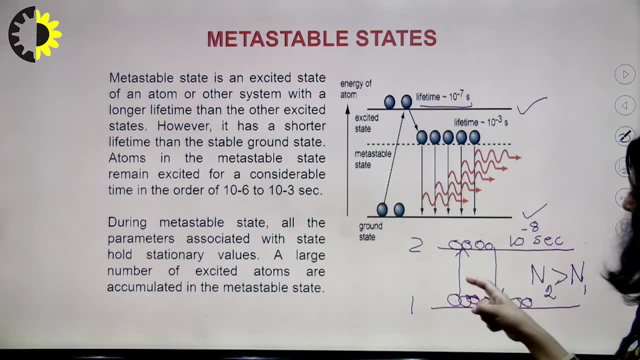 If there are only two states- Ground and excited state- You cannot think about Population version. This state can never be achieved Because the energy- Sorry, Because the lifetime of this state is very small: Atoms which are reaching into state number two. 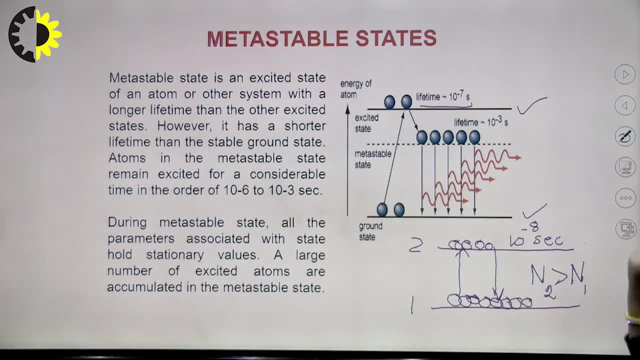 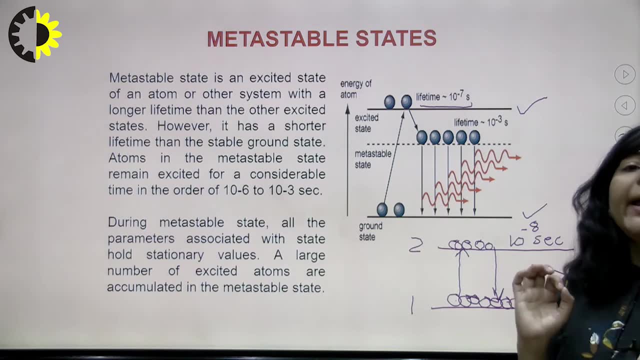 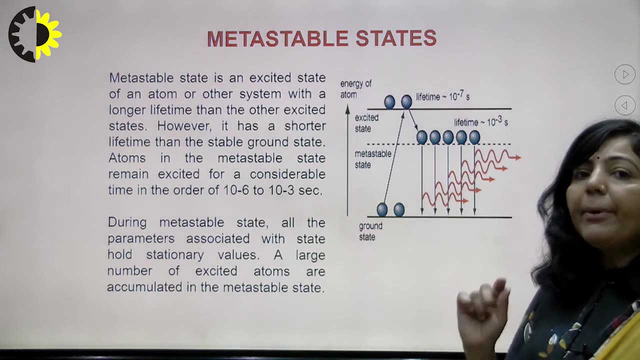 They are not staying there for a longer duration. So you cannot achieve that state Where n2 is greater than n1. So Because of this reason We require an intermediate state. So There should be an intermediate state Between ground and excited state. 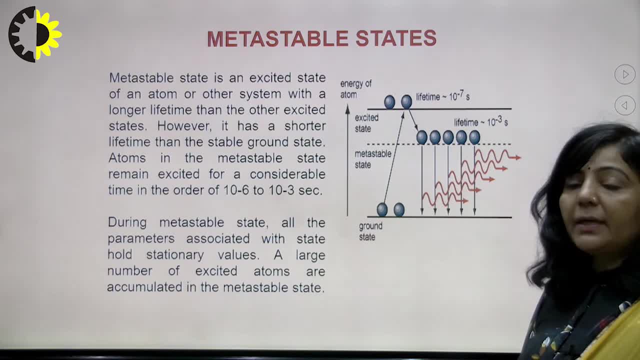 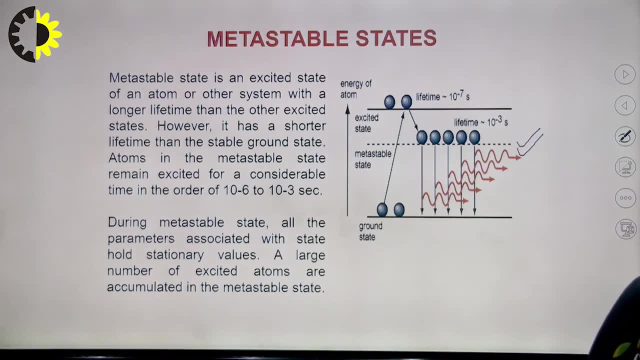 With a longer lifetime As compared to excited state And that particular state. So now we have this intermediate state here. This intermediate state, This state Is having a longer lifetime As compared to excited state And the lifetime of metastable state. 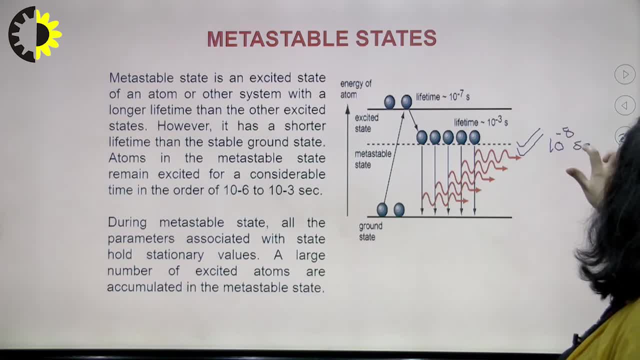 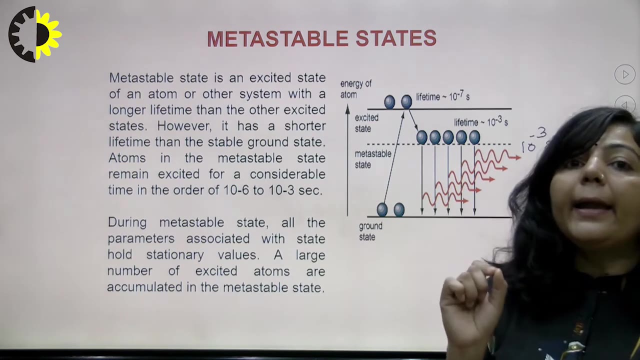 Or that intermediate state Is approximately 10 raise to power Minus. Sorry. This lifetime is 10 raise to power minus 3 seconds. I am so sorry. 10 raise to power minus 3 seconds, So A metastable state. 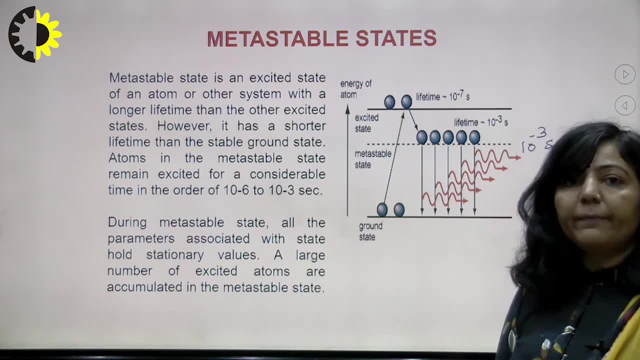 Is basically an intermediate state Between ground and excited state. Now what is the role of that state? That particular state? That particular state Can help us to achieve Population inversion in a laser system If there is no metastable state in between. 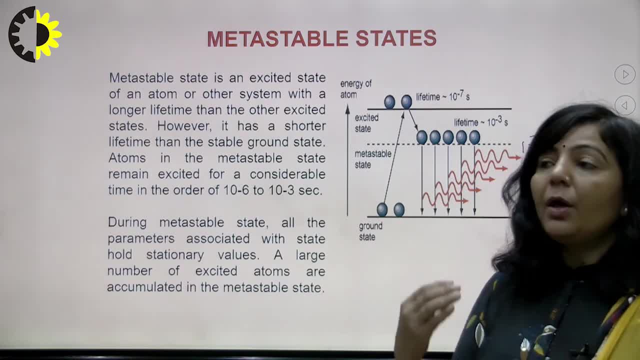 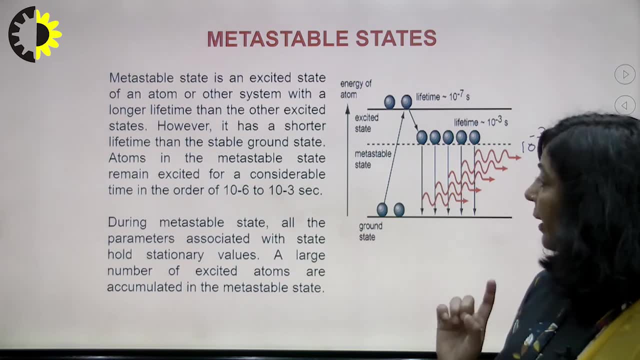 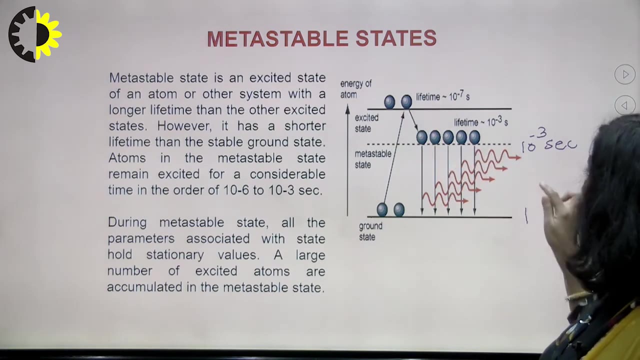 You cannot achieve population inversion Means, you cannot achieve a state When higher, When there are more atoms in higher energy state As compared to ground state. So Exactly what will happen now: From ground state, Atoms will be excited to. 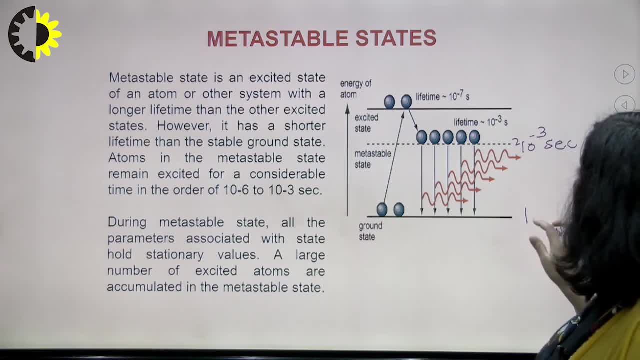 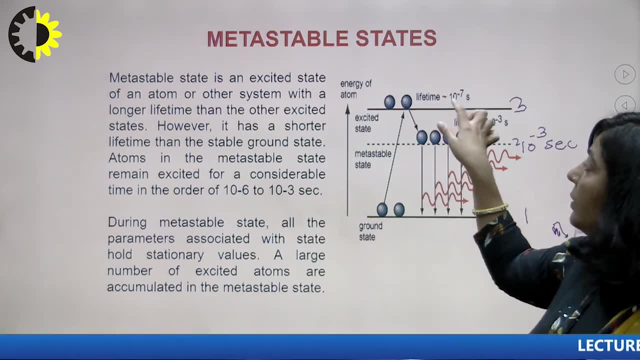 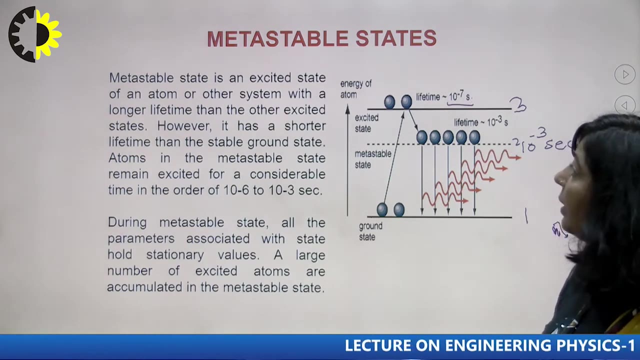 From state number 1. Atoms will be excited to state number 3.. Sorry From 1. Atoms will be pumped to 3. In 3. They will stay for a longer, Sorry for a short duration Of approximately 10 raise to power minus 7.. 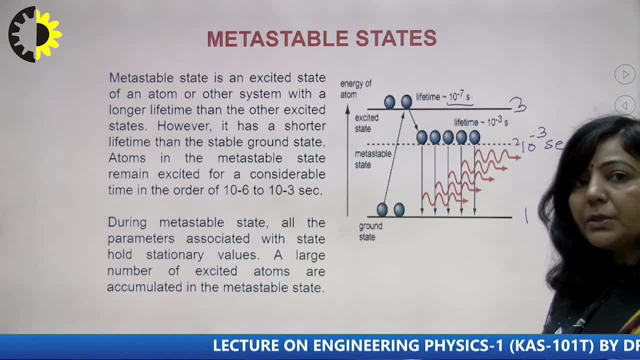 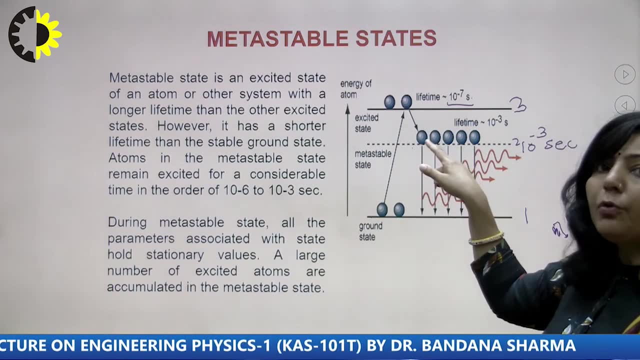 To 10, raise to power minus 8 seconds. After that They will try to come down to a more stable state. So since metastable state is closer to Excited state, So atoms from 3. They will come down to 2.. 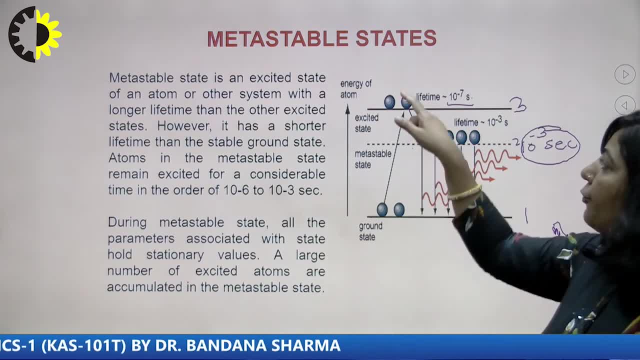 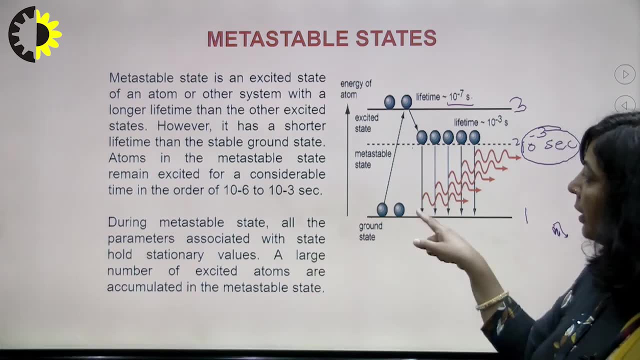 They can stay here for 10 raise to power minus 3 seconds. So from 3. They are coming down to 2. And in 2. They are staying for a longer duration. So exactly what is going on? The population of 1 is decreasing. 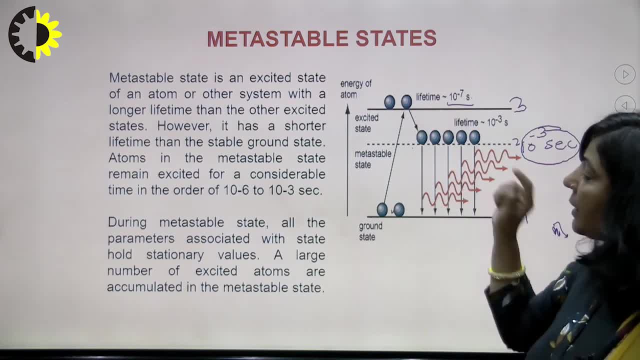 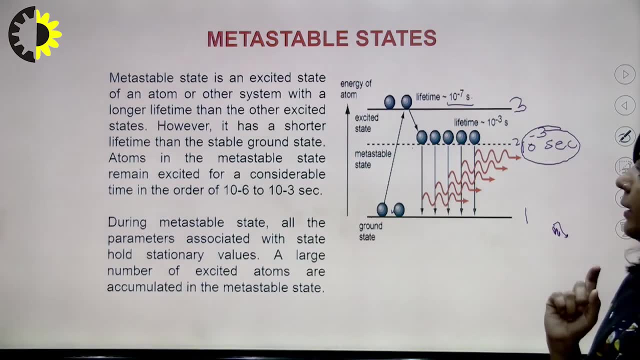 Because from 1. Atoms are pumped to 3.. From 3. Atoms are coming down to 2. And in 2. They are staying for a longer duration. So now you will achieve a state Of metastable state as compared to ground state. 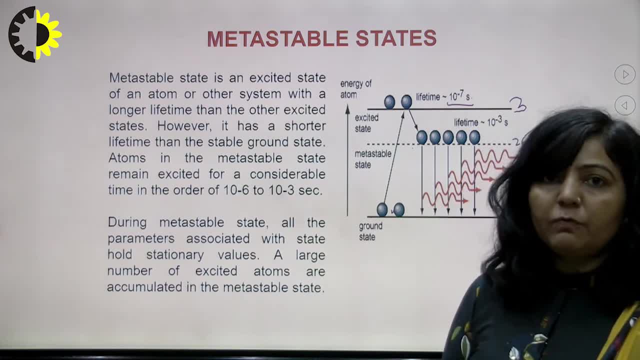 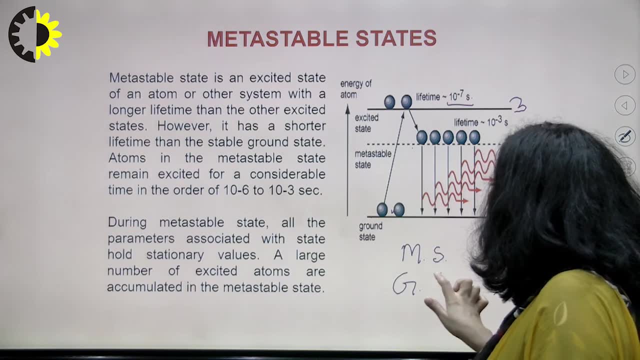 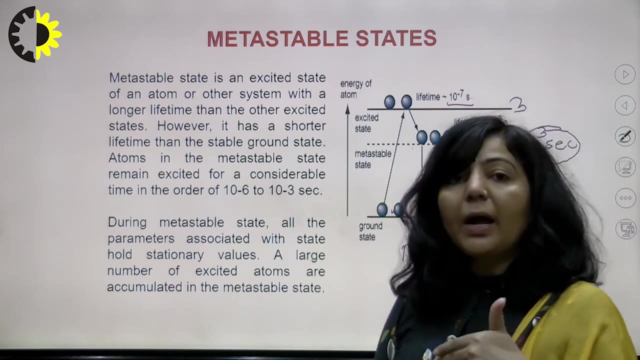 It means Now you are achieving population version, But you are achieving that population version Between metastable state And ground state. You are not achieving that population version Between excited and ground state If there are only 2 states: Ground and excited. 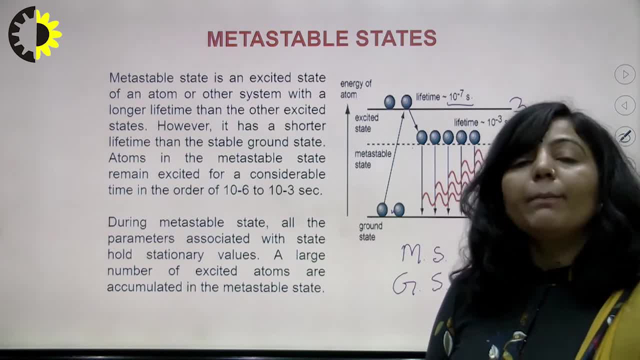 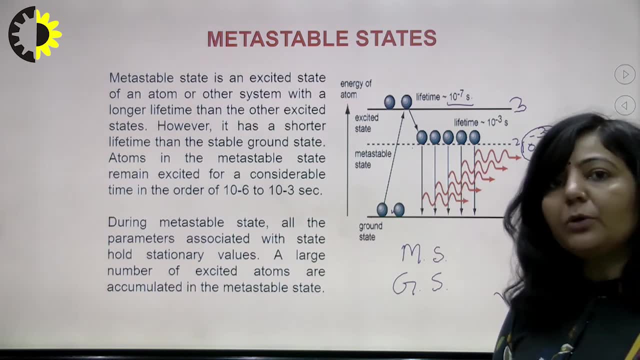 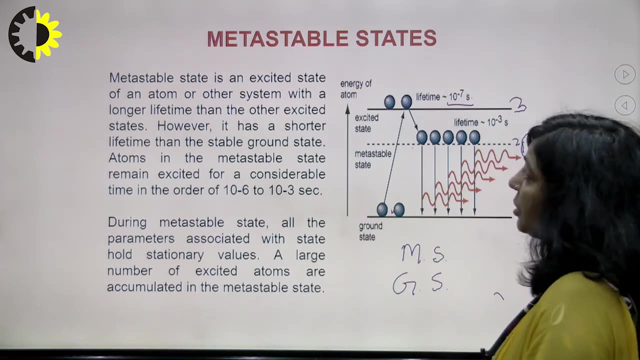 You cannot think about Population version Because that excited state is a very short lived state, So you cannot Exceed the population of that state With respect to ground state. I hope I have made my point clear here Again I am summarizing this metastable state. 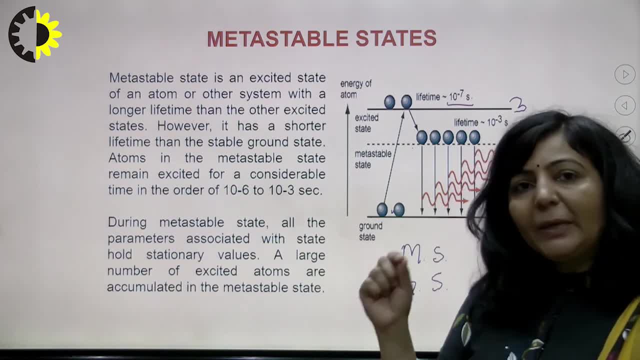 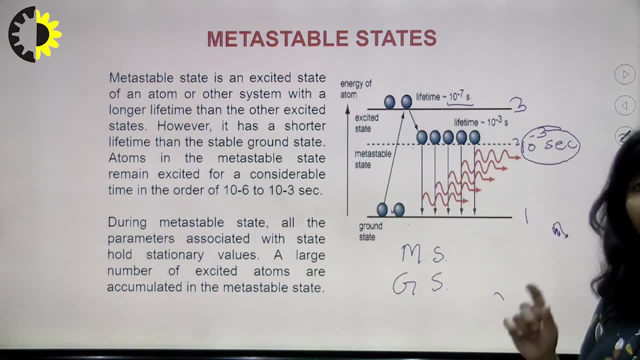 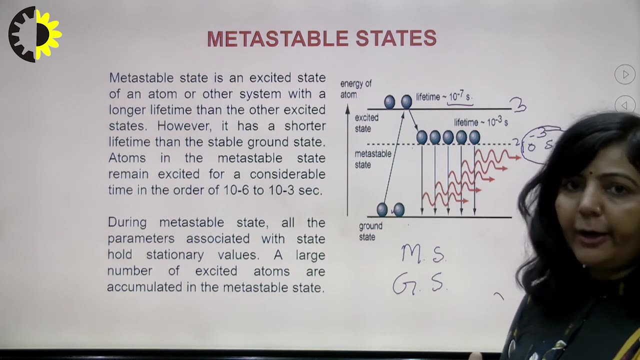 Like this, Metastable state Is basically an intermediate state In between this Ground and excited state, And this state Is having a longer lifetime As compared to excited And it is having a shorter lifetime As compared to ground. 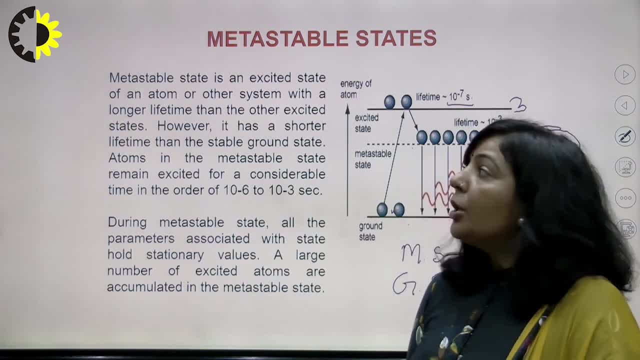 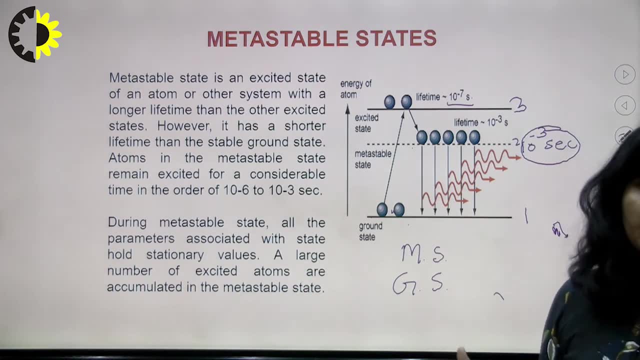 Because ground state is a more stable state. The role of a metastable state, The role of a metastable state In case of a laser Is it is going to help To achieve population version In a laser system. So what are those states? 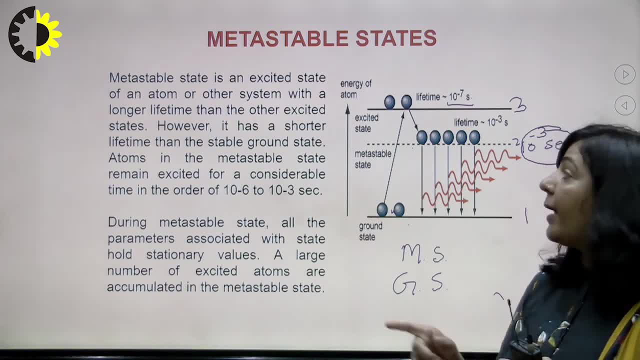 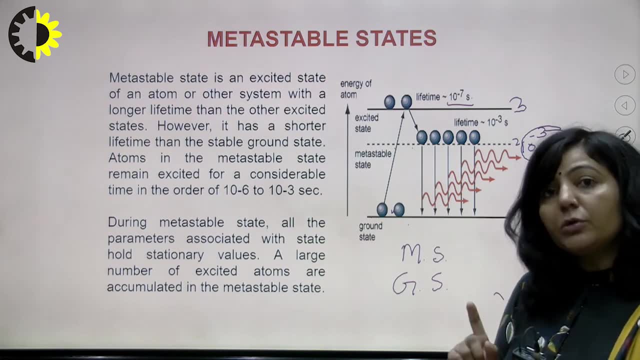 Between which you are achieving population version here. Those 2 states are Metastable states And a ground state. Those 2 states are not excited and ground state- Those states Between which you are getting population version- Is metastable state. 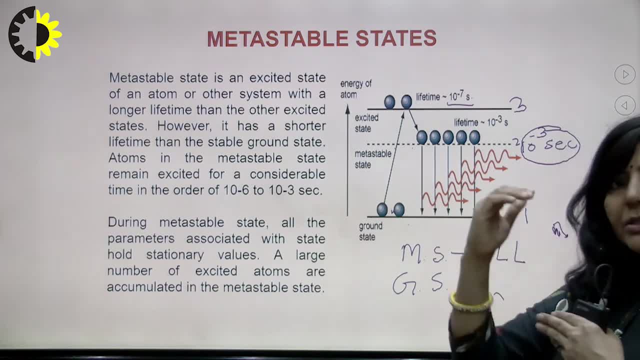 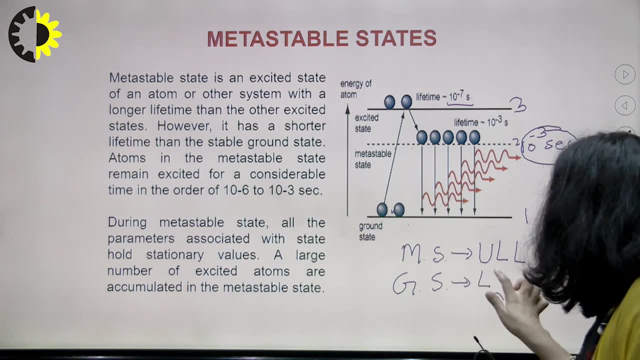 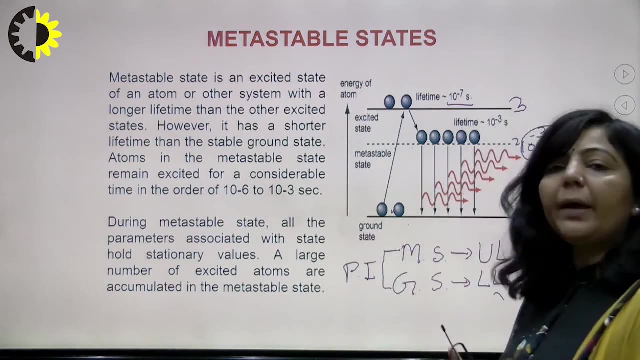 In upper lasing level, The high energy state Which is participating in lasing, And the ground state That will play the role of Lower lasing level, And you are achieving population version Between these 2.. Right, So these are your metastable states.